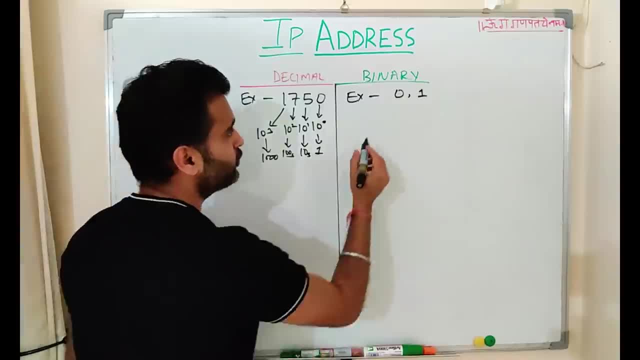 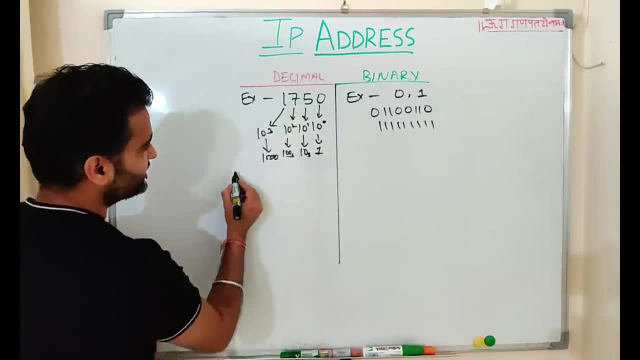 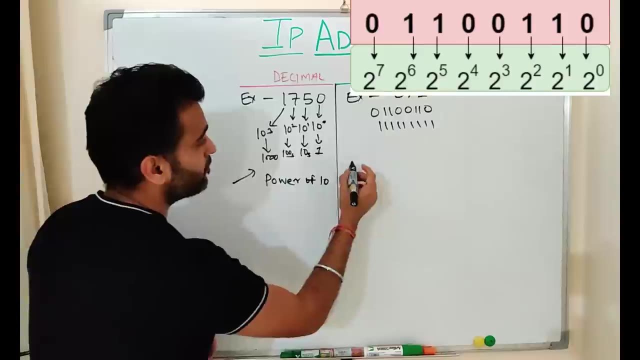 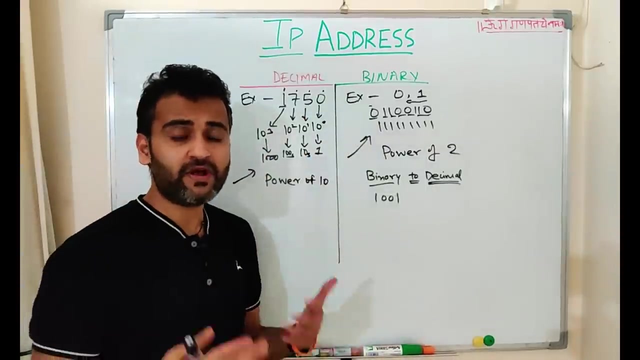 or 1. so any number which you see in binary would be of this nature or like something like this: so this, this particular, uh, decimal numbers are power of 10, but in, in binary, we have power of 2. so, friends, now, as we know that binaries are power of 2 and the decimal numbers are power of 10, we 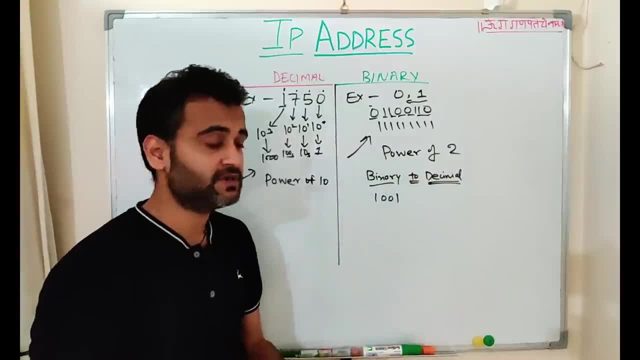 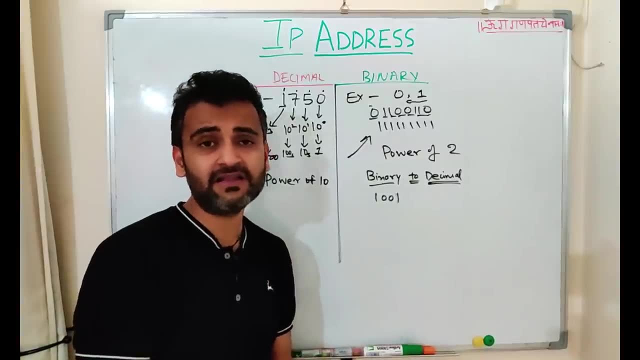 will quickly try to convert a binary into a decimal. so, friends, i am just explaining this concept so so that you better understand how ip addresses exactly work, uh, underneath. but in case you already know this, you can skip this section and directly move on to the ipv4 section. so in 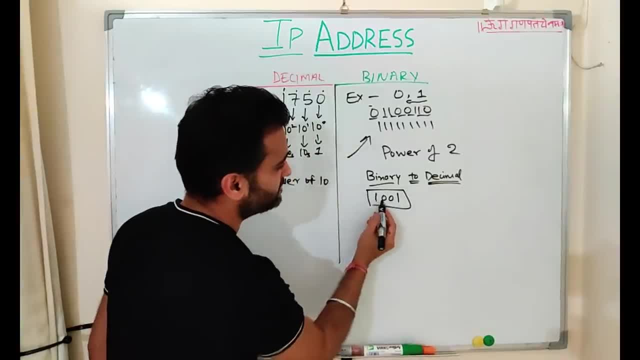 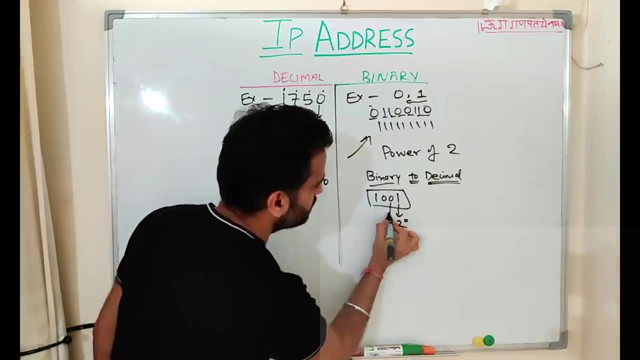 this case, let's ex, let's take an example of this binary: number one: zero, zero one. so we will simply write it like this: so this is 2 to the power 0. this is 2 to the power 1. this is two to the powers. 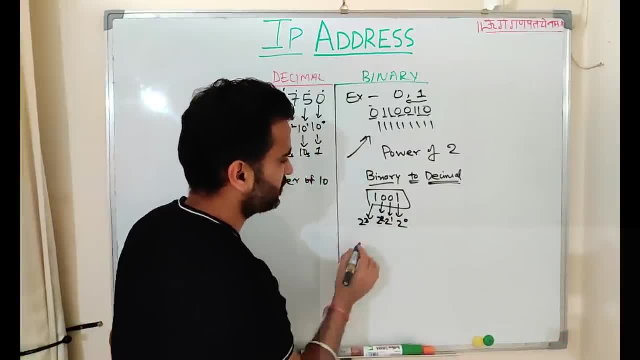 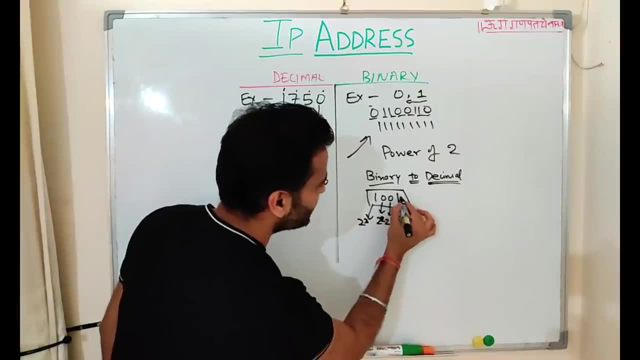 two, and this is two to the power. three, okay, so we will add these equivalents. so what is this? so it is 2 to the power 0, and what is the exact number here? one, so it would be 2 to the power 0, 1. 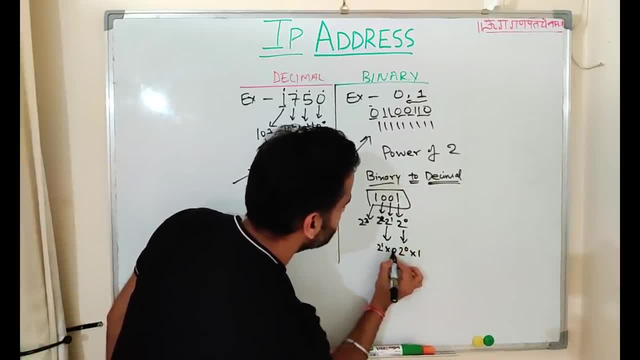 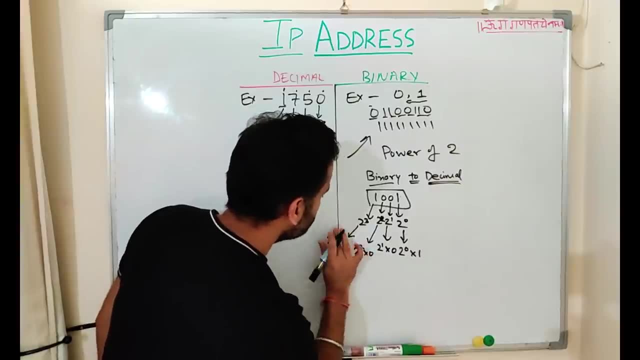 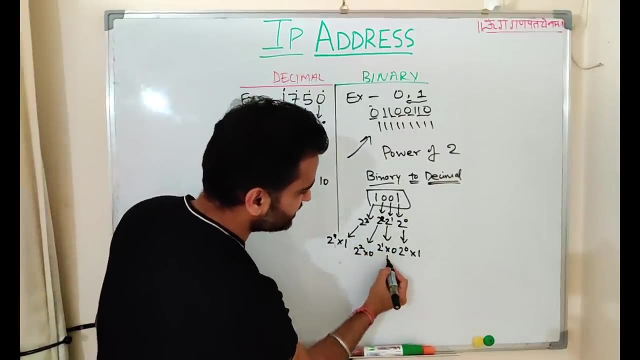 this would be two to the power, one into zero, this would be two to the power, two into zero, and this would be two to the power, two to the power, three into one. now, wherever there is multiplication with zero, okay, this would be simply zero, but wherever this, 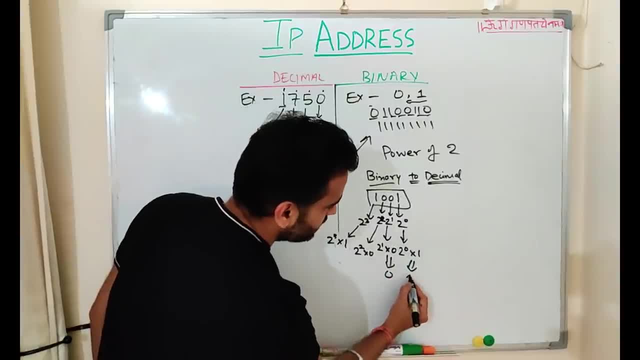 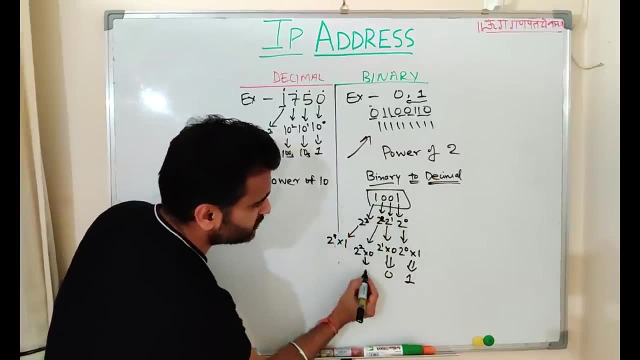 is one. so two to the power zero is one, and one into one equals to one. here it is two to the power two, which is four, but it is eventually getting multiplied with the zero, so it is also zero. and then, here it is two to the power three, which is eight. two into two into two, which is eight. 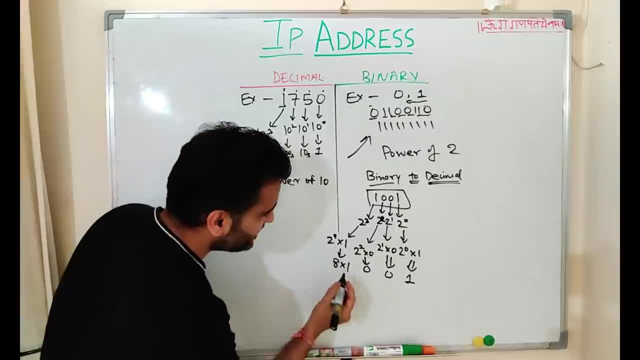 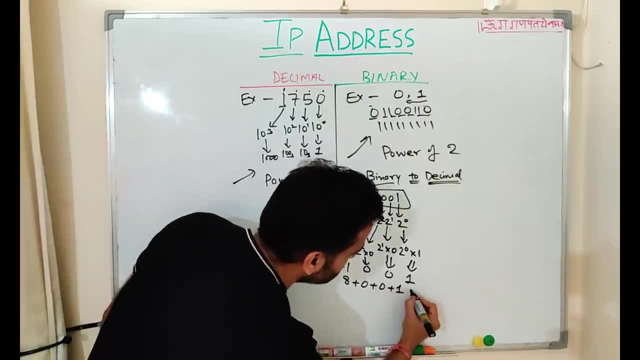 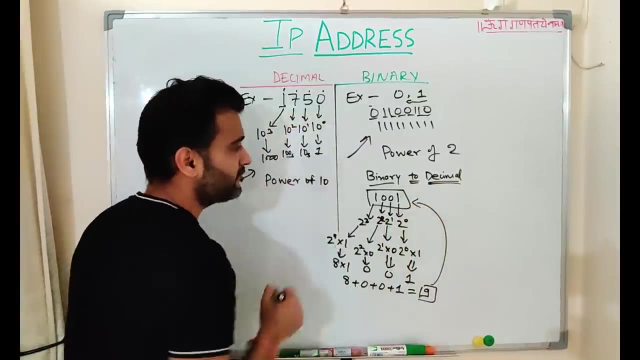 so here it is eight into one, okay, which is exactly eight. so what? what is the total sum? eight plus zero plus zero plus one which is nine. so nine is the decimal equivalent of this binary: one zero zero one. so, friends, as we now know how to convert a binary to a binary, we can convert a binary to a. 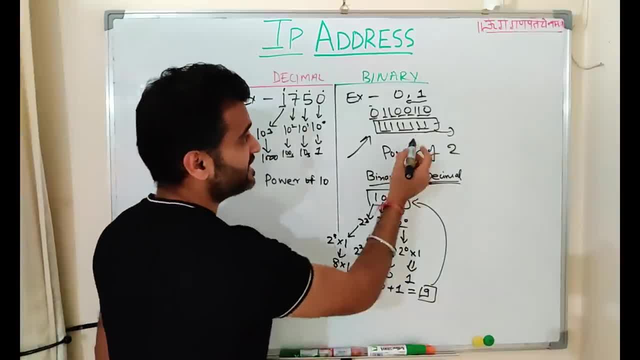 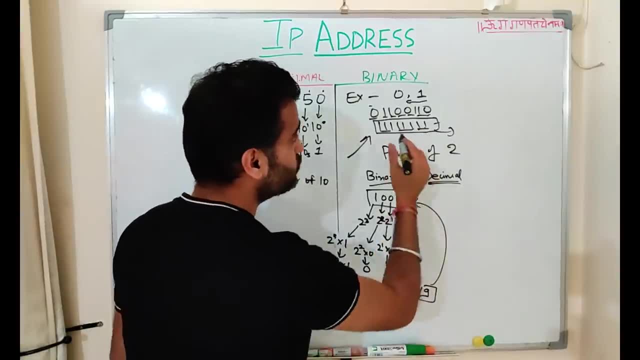 binary by using a binary. so let me show you how to convert a binary to a binary by using a binary binary into decimal, just understand. once again we will recap that every entity within a binary number is either zero or one, and then this is called as a bit okay. and when you combine 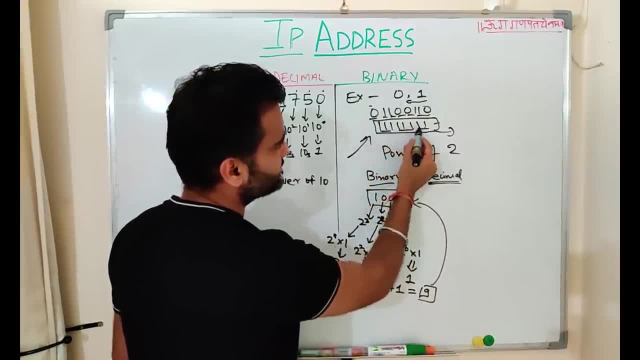 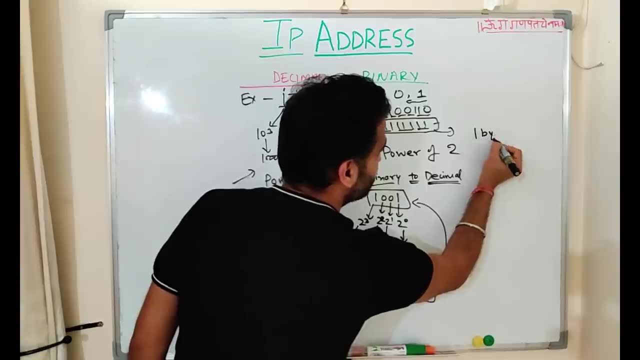 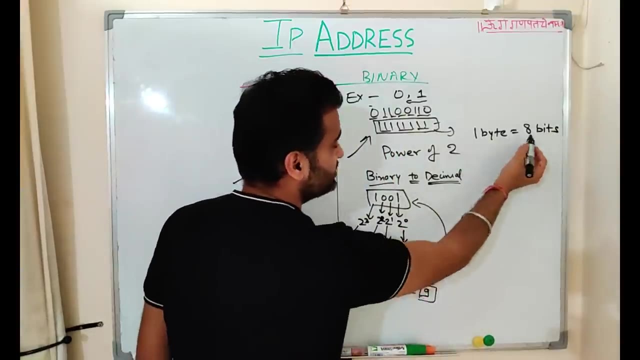 eight bits. so in this example we have eight bits: one, two, three, four, five, six, seven, eight. you can either have zero, you can have one, so in this we have eight bits, so eight bits. so one bite equals to eight bits. okay, and then this particular combination of eight. 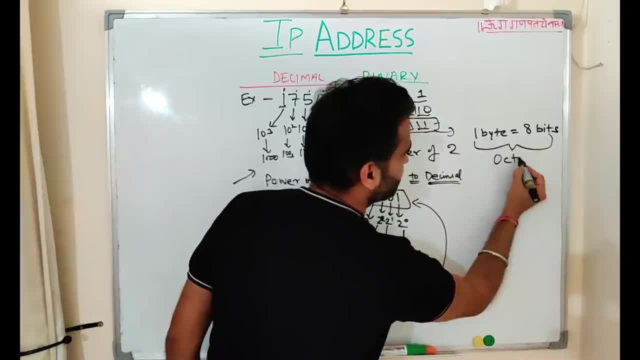 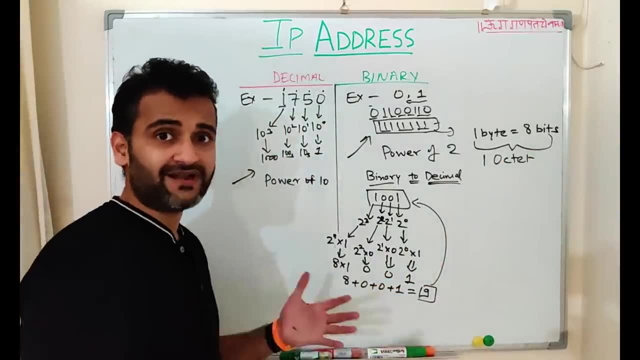 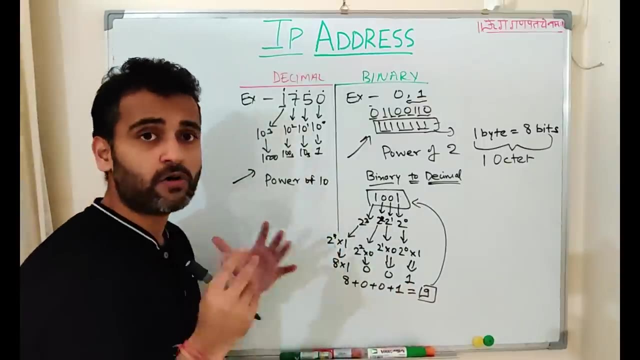 bits is called an octet, so this is one octet. okay, one octet is a combination of eight bits. you will understand this once. we will now cover this into ipv4 section. okay, so let's move on to the new and next section. we now know a. 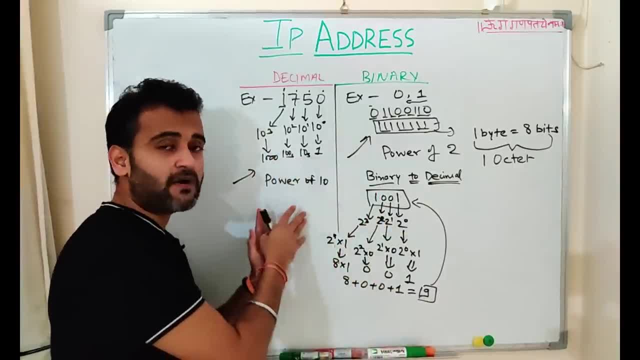 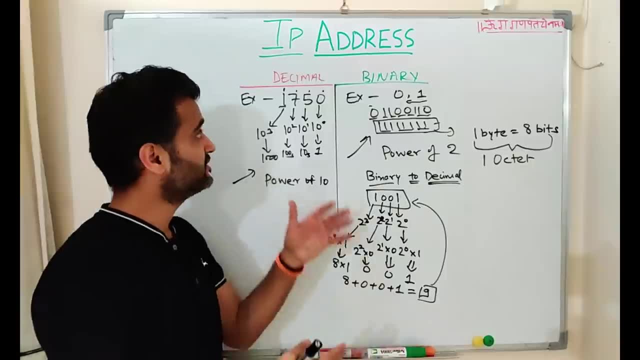 basic order, order, order over here, which is of what is a decimal number, what is a binary number? this is power of 10. this is power of 2. how to convert it? here it is called as digits. here it is called as bits and bytes. this can. 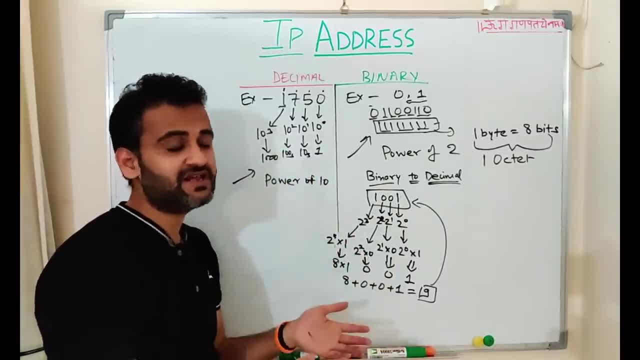 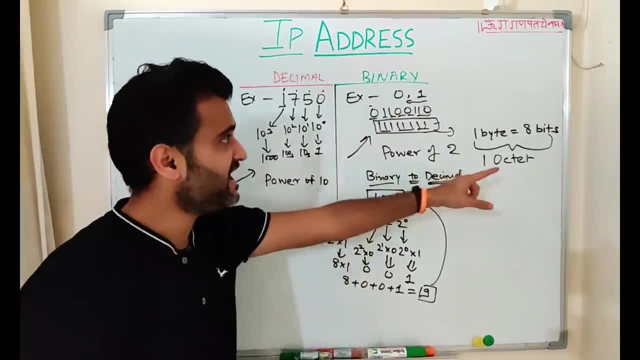 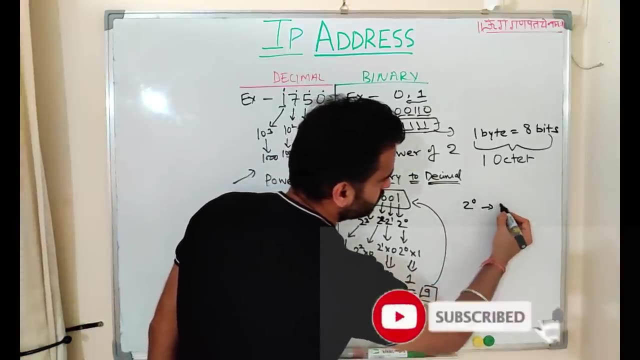 be. you know tens, hundreds, thousands, millions. here it can be. you know only the power of 2 and only 0 and 1. okay, so the maximum in an 8 bit, how much you can have in 8 bit? so it can maximum be from 2 to the power 0 to 2 to the power 8, so this comes out to be maximum. 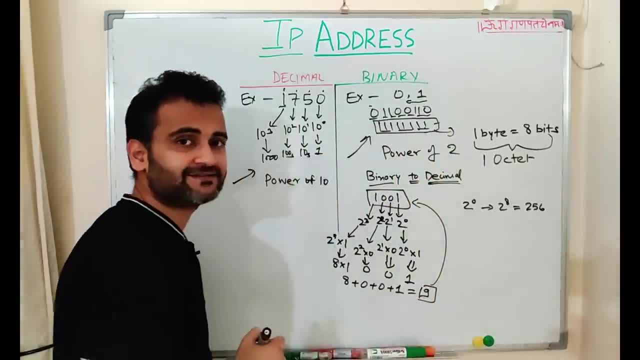 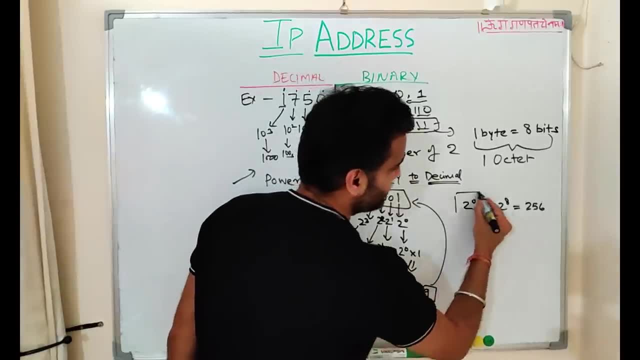 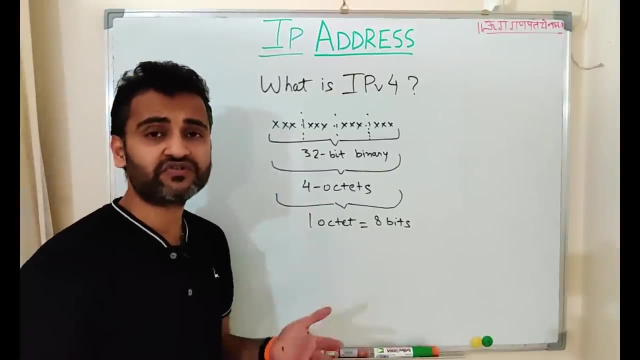 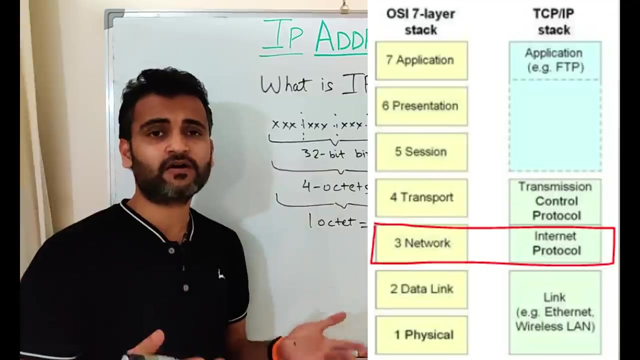 of 256, so we can have 256 different combinations of numbers within this range. so now let's understand what is IP v before? so ipv4, which is an IP address, version 4 resides at the next network layer of our TCP IP model, and any device which is there on the network needs to have this. 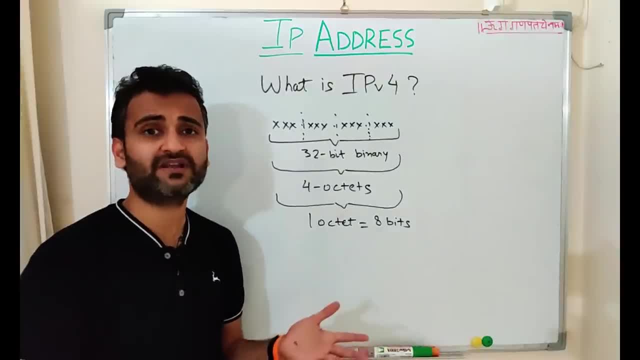 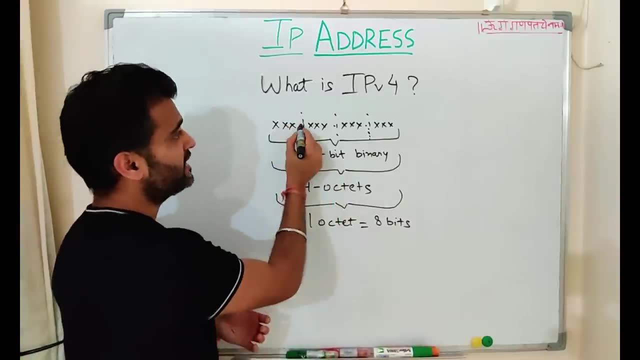 unique identity, this unique address to be identified over the network. so what is an IP address? so IP address is something like this: you know you will have some decimal number, so and it there would be a dot in between, so what it is called. it is called as dotted decimal. 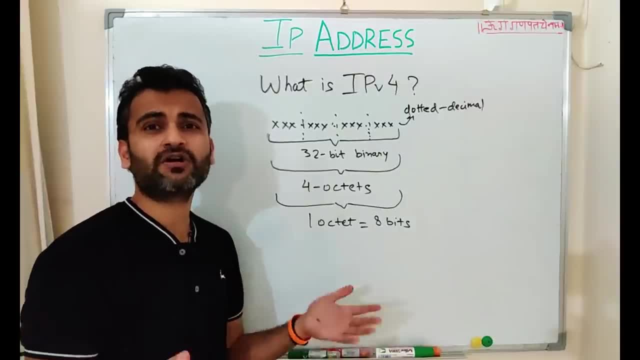 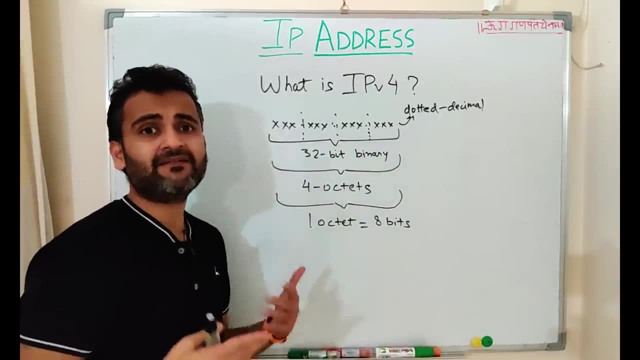 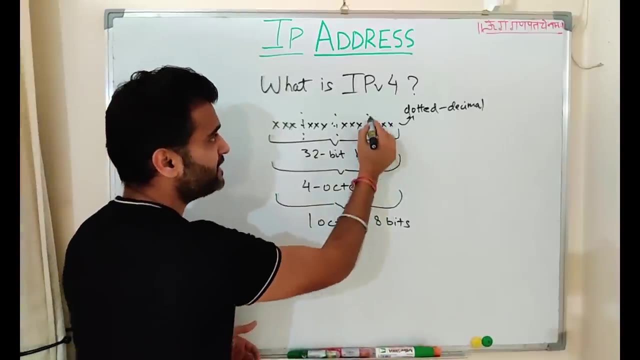 so an IP address is always shown as a dotted decimal number. okay, so every you know, every decimal number underlined is a binary bit. so basically what you have, you have a 32-bit binary. 32-bit binary. how? because every section here is kind of an octet. what is an octet? I told you. 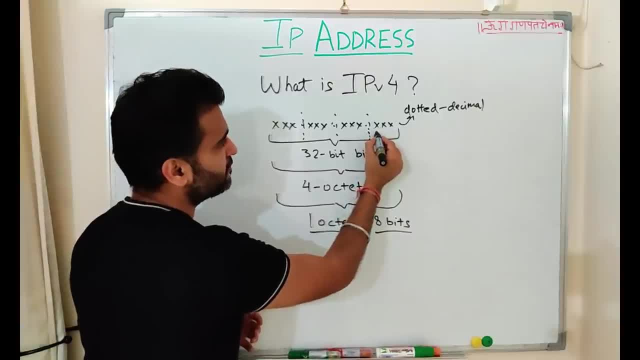 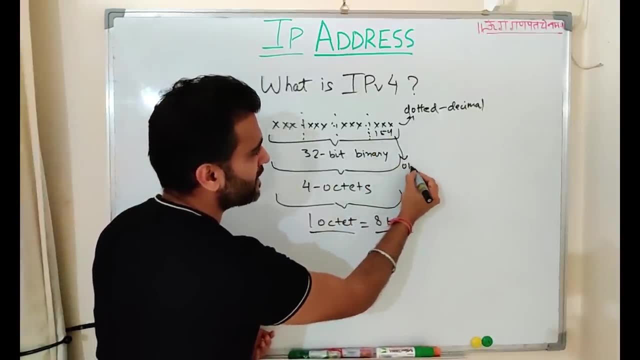 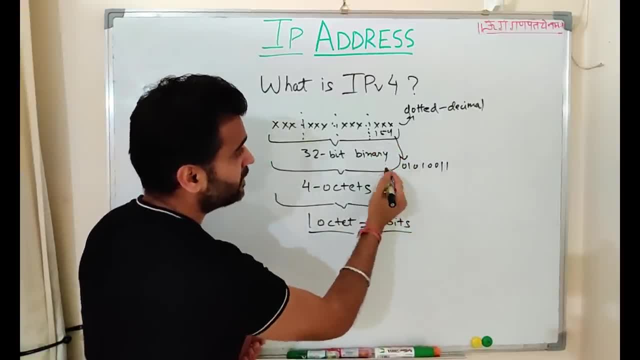 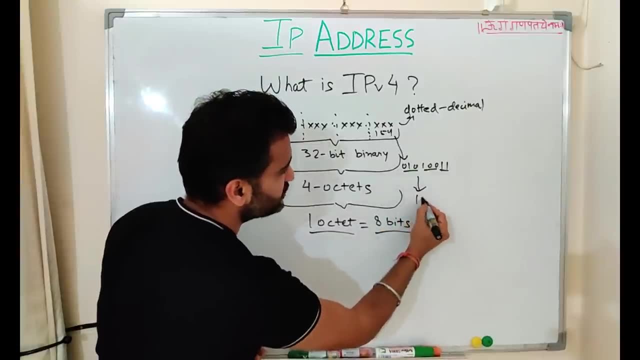 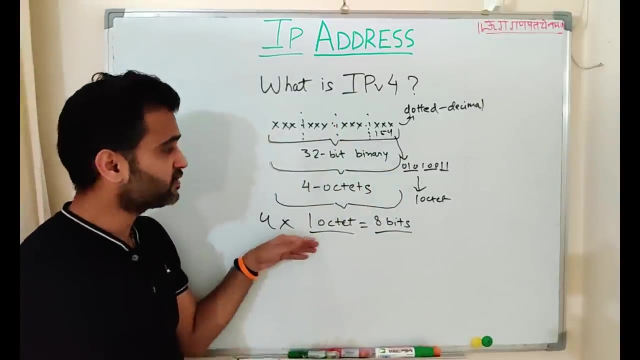 I am just giving you an example, because it will take too much time. so this 142, 54 is kind of a combination of 8 bits. now, combination of these 8 bits is one octet. okay, so when we have four different octets, so if we multiply these into four, four octets, then this is regarded, regarded. 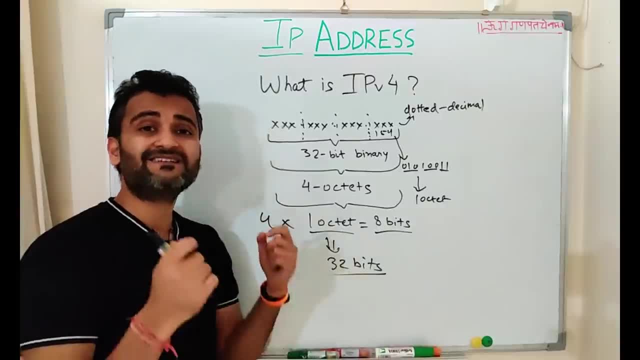 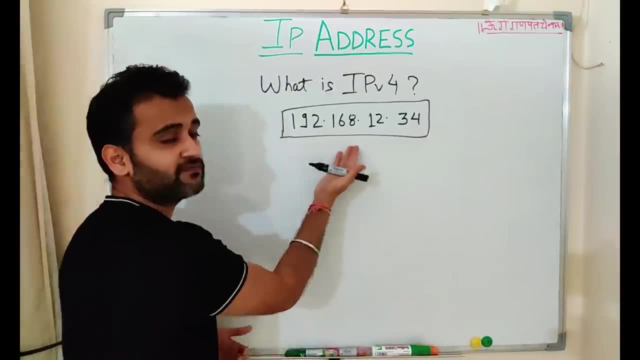 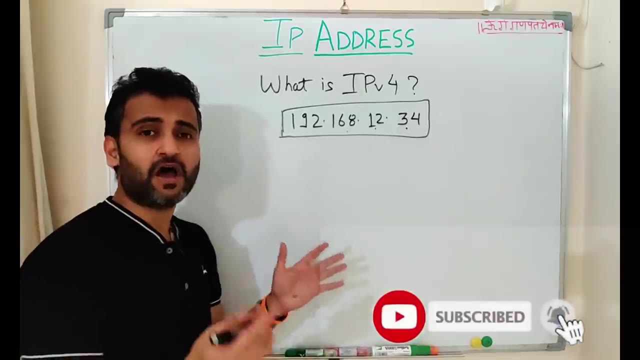 as 32 bits. so every IPv4 address is a 32-bit logical address. now let's move ahead and understand more about IP address. so suppose take, for example, this is an IP address 192.168.12.34. so this particular IP address- any IP address for that matter- will always have two parts. okay, don't take it in this. 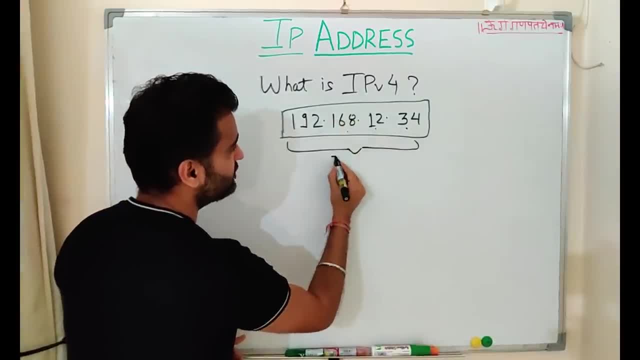 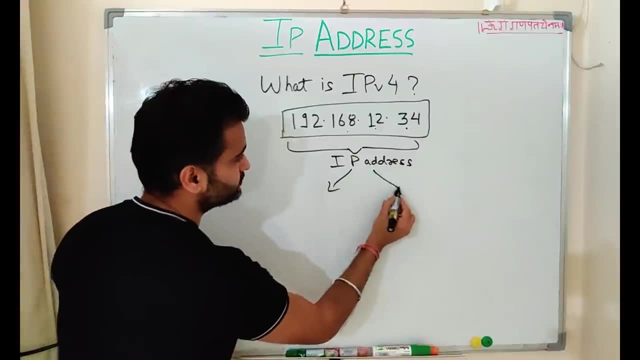 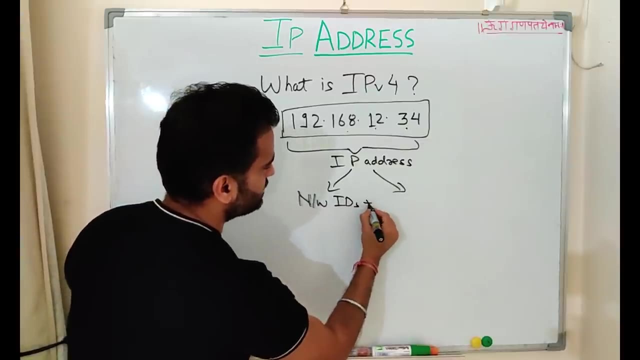 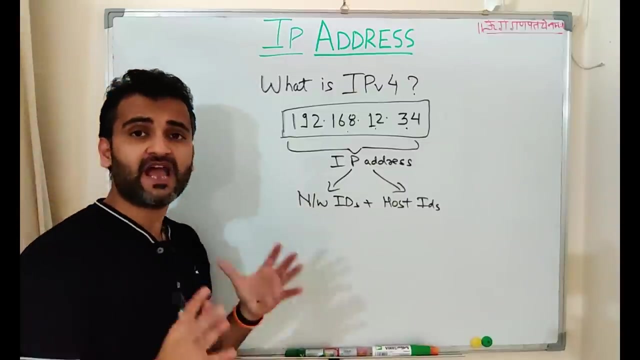 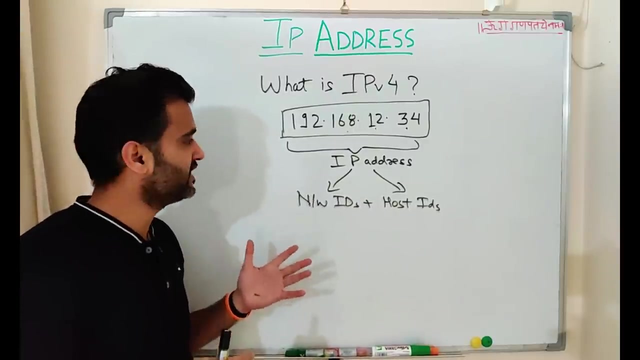 way. but just understand that if this is an a total IP address, then it will be divided into two parts. okay, so it will have network ids and then it will also have host ids. okay, so every, every IP address will have two parts. but how you segregate that, that depends on the next topic which we will take up quickly, that how, how much. 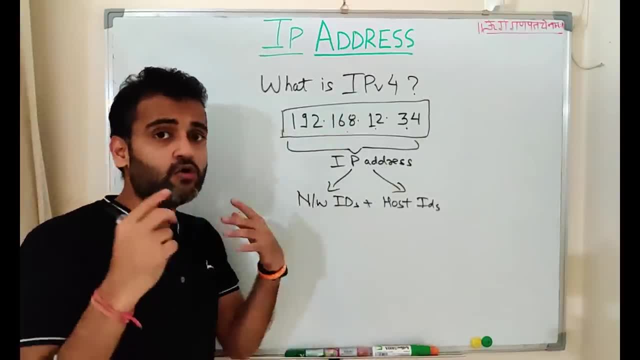 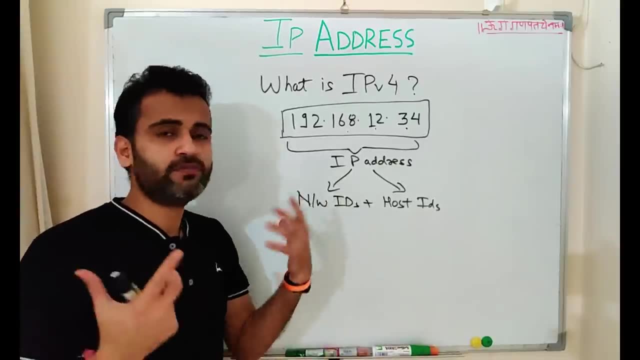 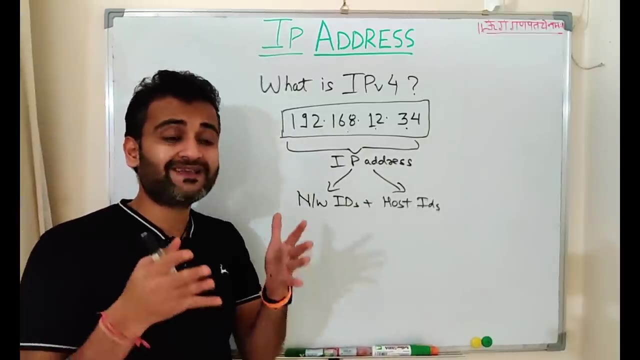 part of a IP address should belong to network and how much part of an IP address should belong to the host. so what is a network? so any device which is connected will be connected to a network, right? so in that particular network, how many IDs you would want to distribute to exactly help the? 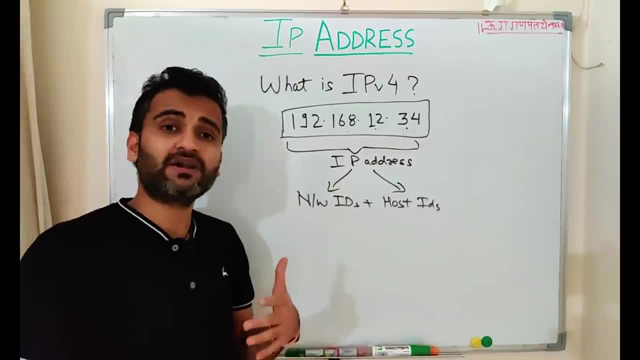 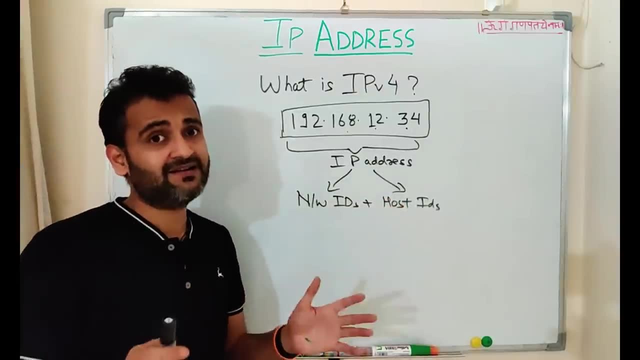 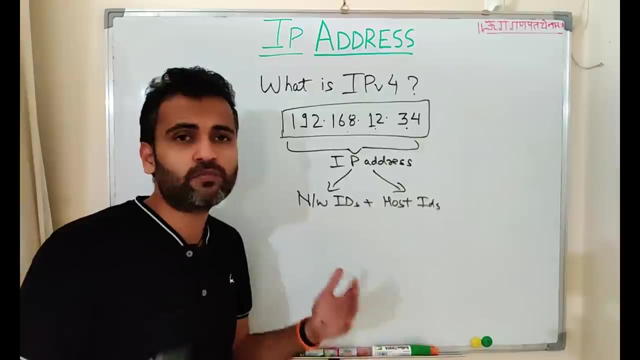 network. you know, do the communication part, but then you have to also distribute specific IP addresses to the host. and understand this, guys, that you know we only have limited IP addresses. okay, we will. we have around four billion IP addresses, if I am not wrong, and these you know. 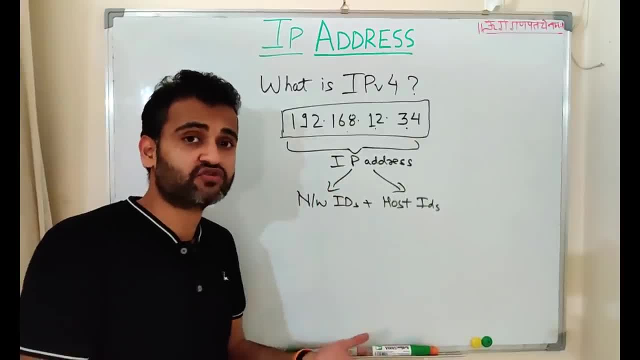 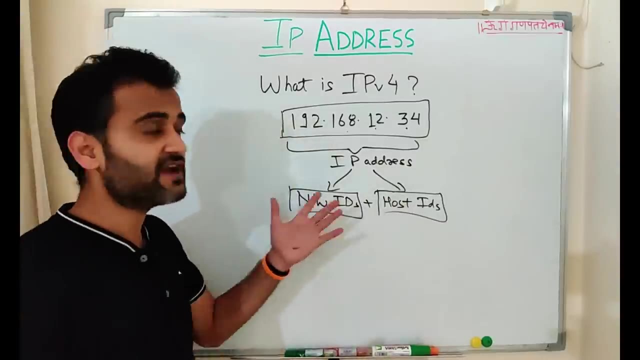 IP addresses are definite in numbers, so it would exhaust. so we have to judiciously use these IP addresses. okay, and that is where we will discuss ipv6- why- why we need ipv6 in the later part. but understand that we will always have network IDs and host IDs to take for example this particular. 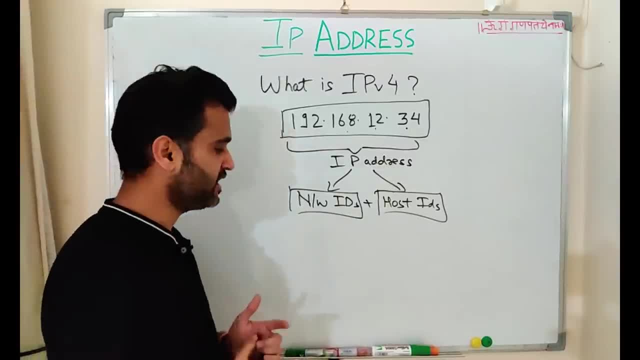 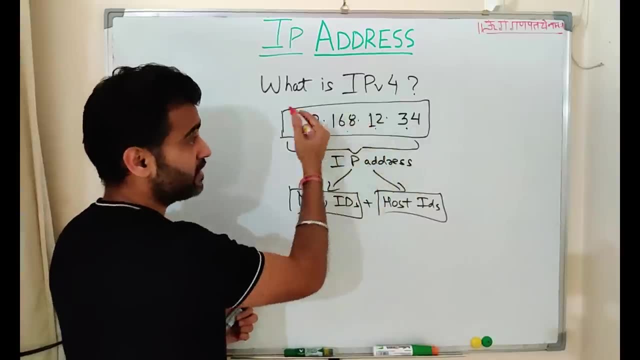 you know, if this particular IP address we take, then in this particular IP address and don't take it on my, on this particular IP address. but I am trying to explain and I am trying to explain and we will discuss this later also, this particular part could be network and this could could be the 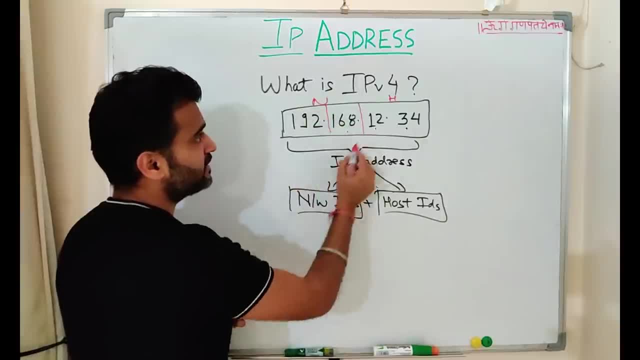 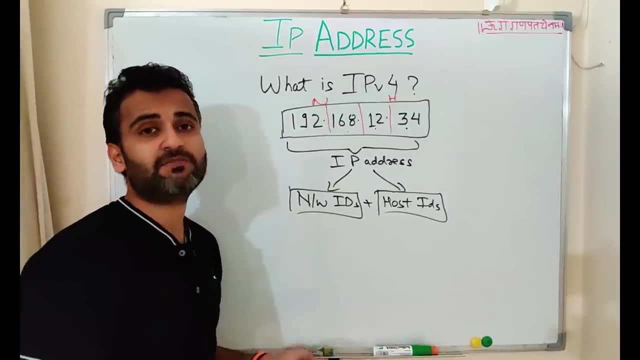 host. okay, but how to divide it? it could be divided here. it could be divided here: where, where we have to segregate that that is dependent on the class of that IP address, we in which particular class that particular IP address belongs, because that helps us to understand how we have to utilize is. 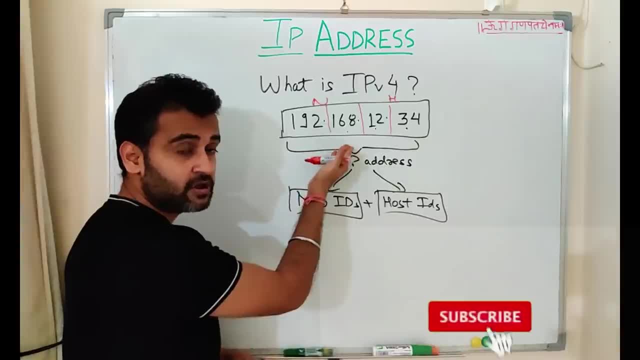 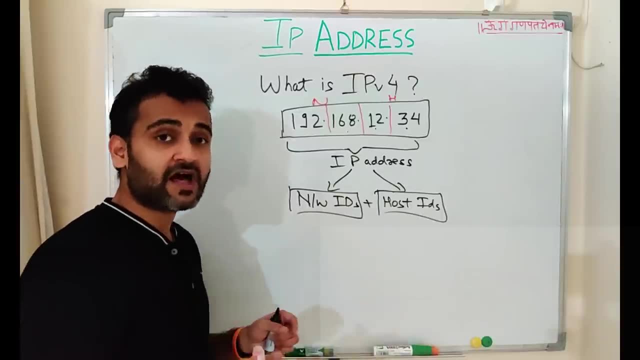 if the network- do we need more network? or we do we need more network, or do we need more network or host? that is a call which is derived from understanding which particular class this particular network belongs to, which is our next topic. so, friends, now we will understand what are. 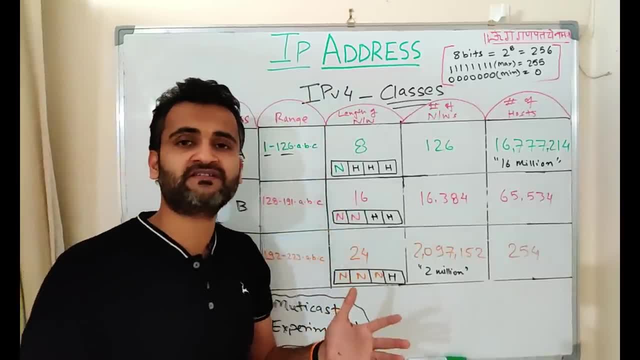 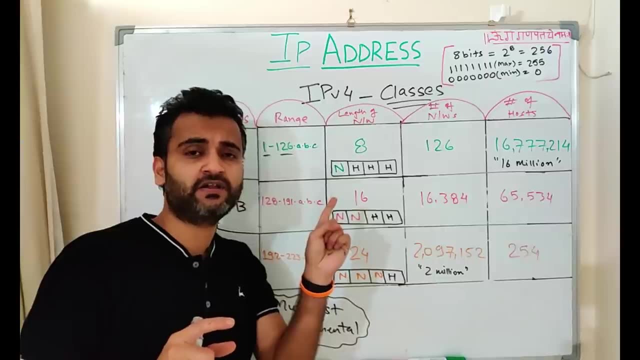 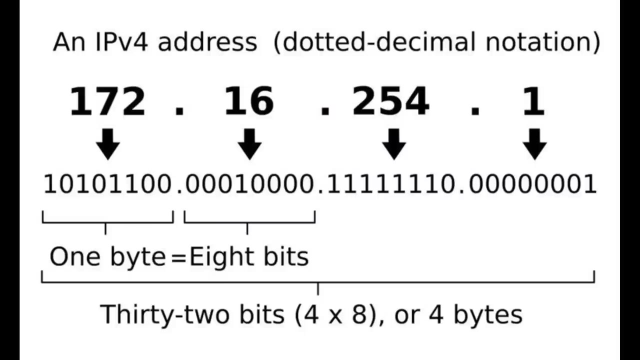 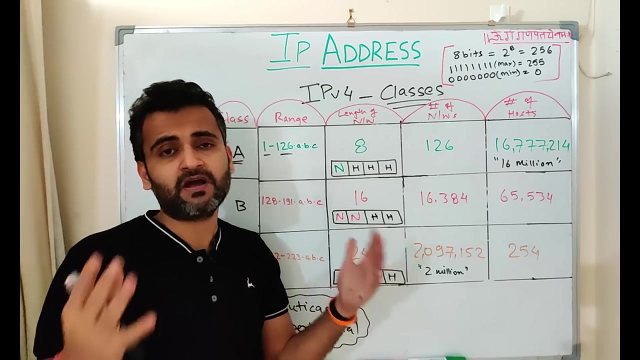 different IP v4 classes and how IP addresses can be categorized within these classes. but before that, a quick recap of our binary section video, so that we understand some basics. and recap it, one byte is equal to eight different bits and those combination of eight bits forms one octet and one particular octet. you know, when multiplied by four that means 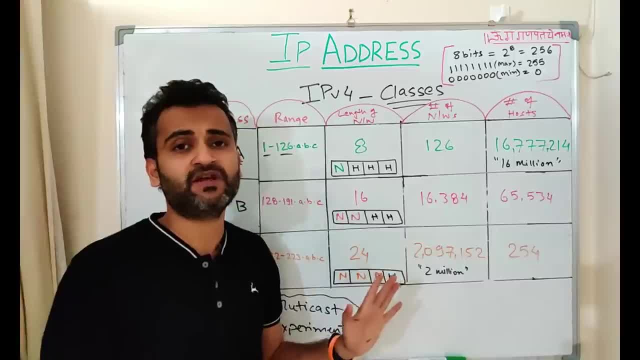 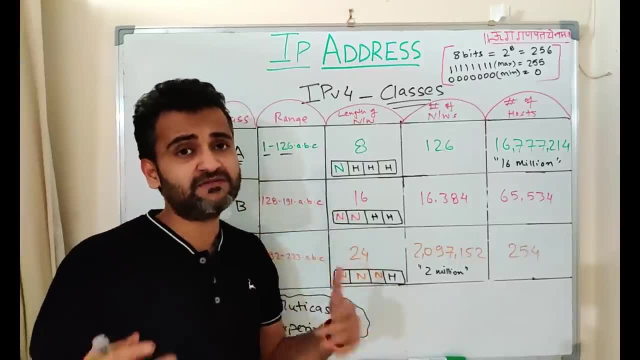 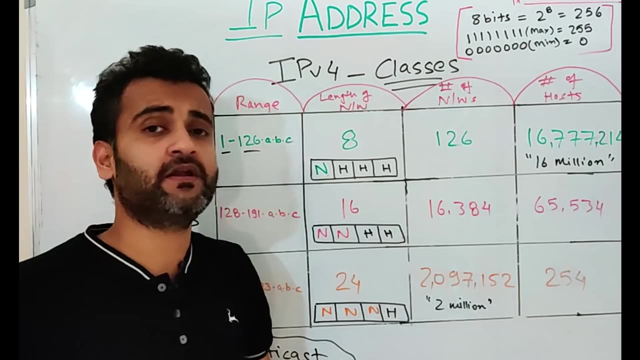 four different octets when comes together creates a 32-bit IP address. so you can understand the hierarchy now, combination of eight bits means power of two, as I told you. so two to power eight, we can have 256 different combination of binary numbers within one particular octet or one. 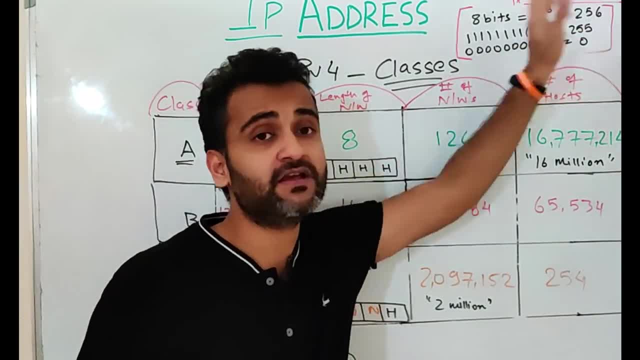 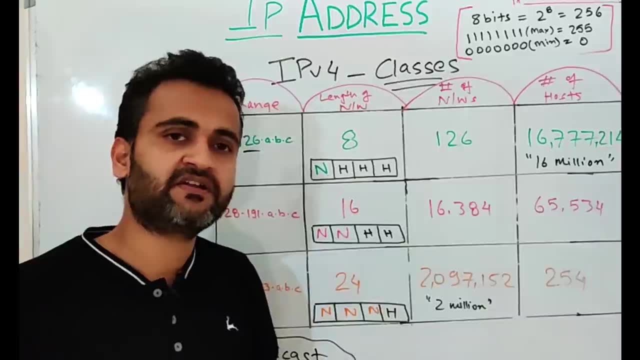 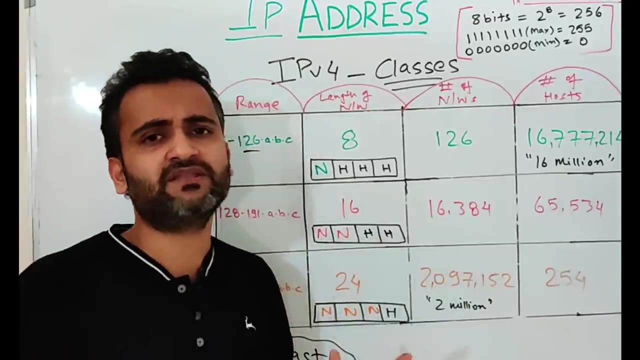 particular byte or eight different bits, so two to the power eight, which is 256, so 256 different combination of binary numbers can reside in eight bits equivalent to one byte and also equivalent to one octet. take, for example, to correlate it with a decimal number. take, for example, if there is a number. 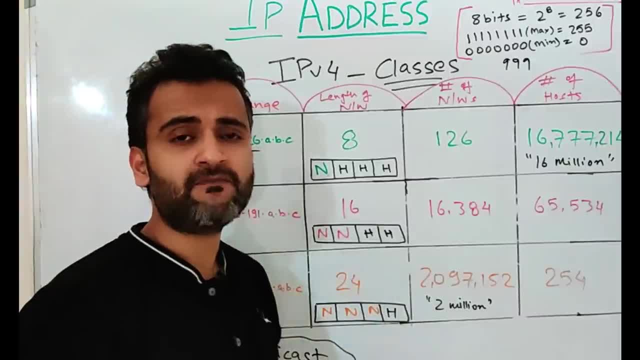 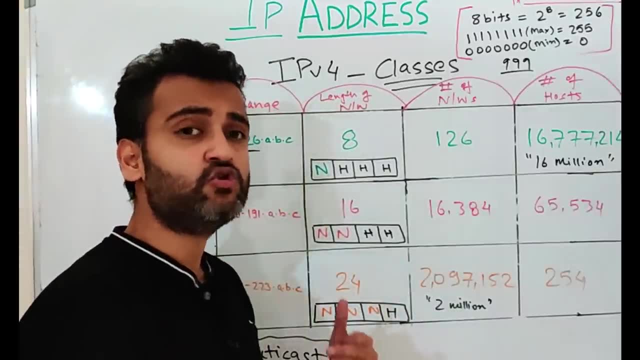 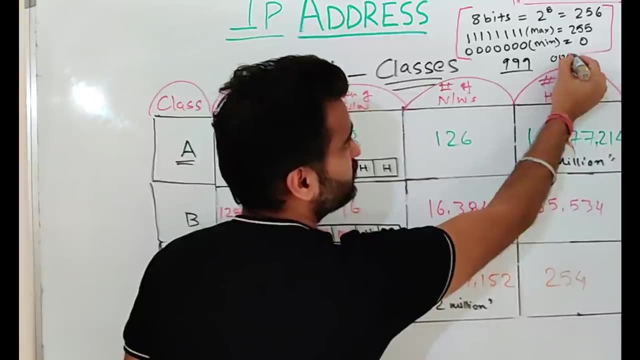 called as nine, nine, nine. so the maximum value which you can store here is a 999. okay, but at the same time you can have thousand different combinations of numbers which can reside in this. so you can have, you can start from zero, zero, zero. one, two, three, blah, blah, blah. 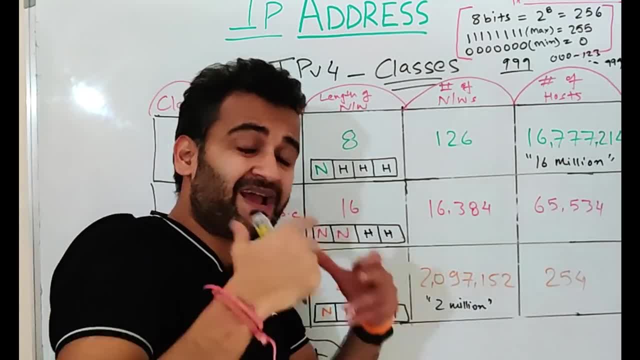 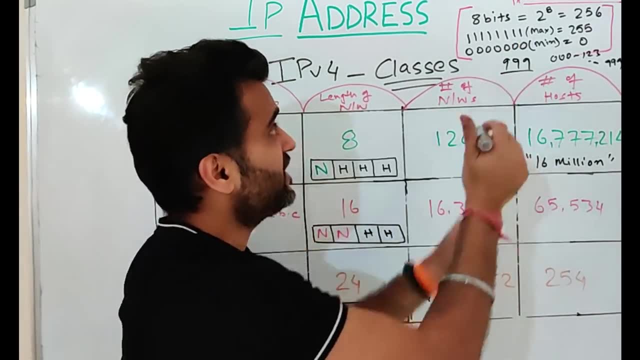 ending up to nine, nine, nine. so there is a difference maximum value. what you can store is 999, which in case of you know a binary number. if you take binary and if you make everything one, okay, so the maximum you can store is 255 and if you keep everything zero, then you can store 255 and 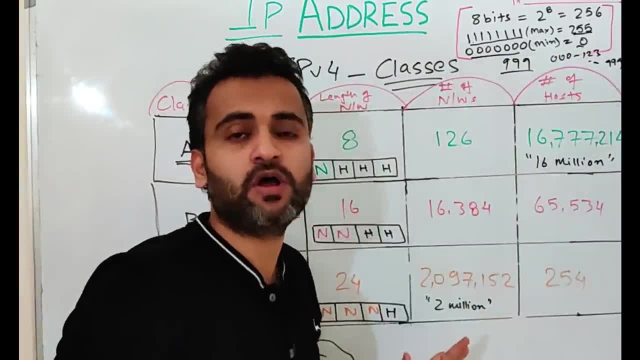 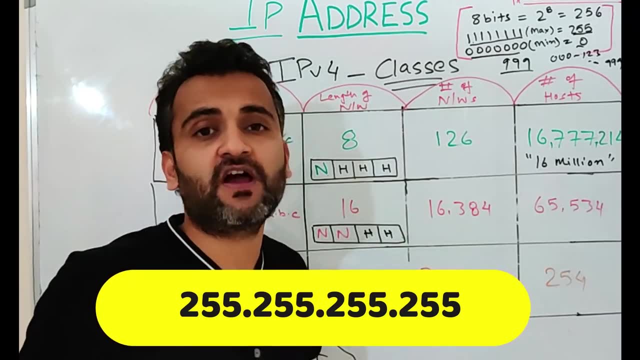 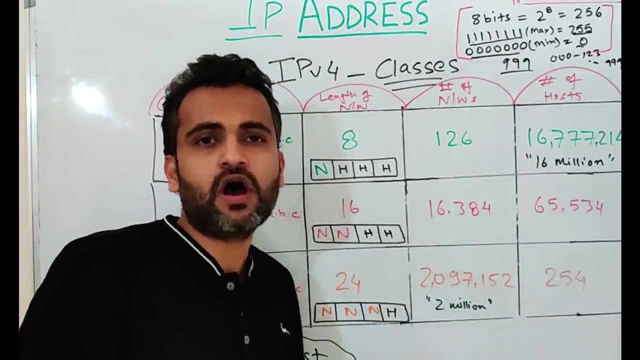 if you keep everything, zero is you know it will be zero. so what could be the maximum ip address you can have? you can have 255.255.255.255. every address which you see should be. you know should be within this range. so 0.0.0 up till 255.255.255.255, because that is the maximum you can. 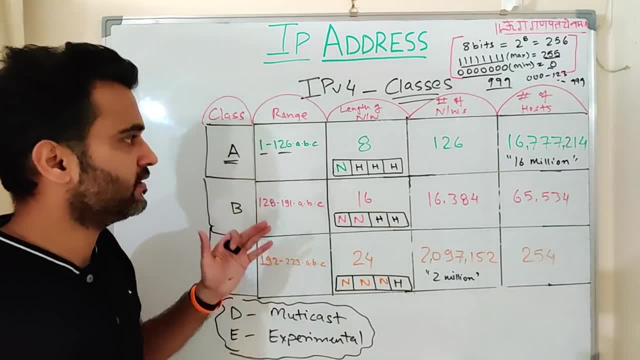 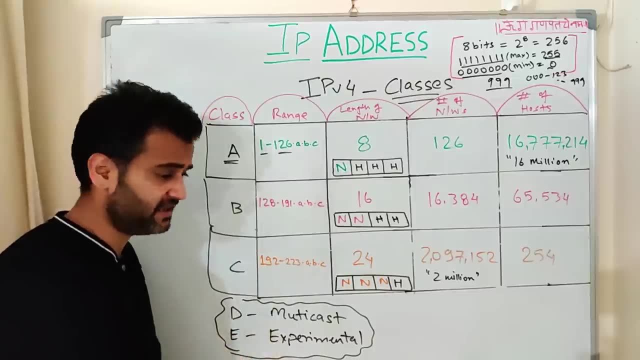 reach right understood. now coming back to our different classes, so basically we have five different classes of ip address: class a, class b, class c, class d and class e. so let's start with class d and e, because these we will not discuss in detail. so basically we have divided the ranges. 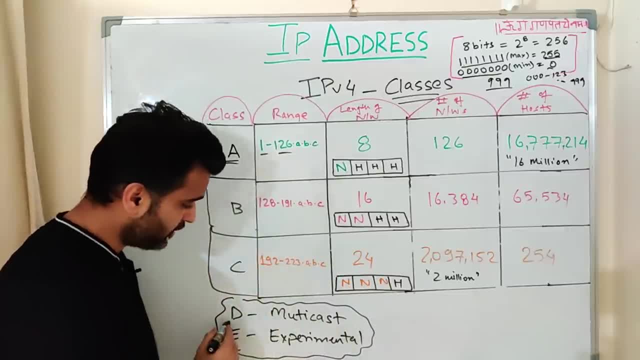 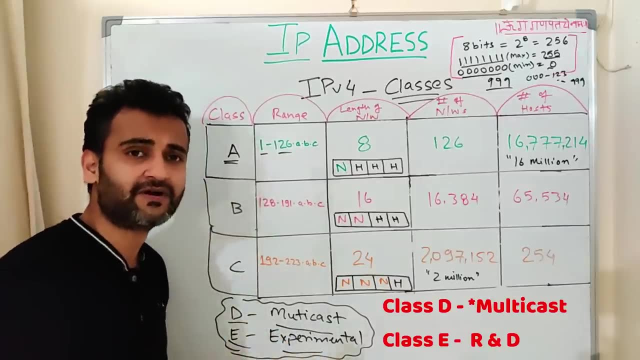 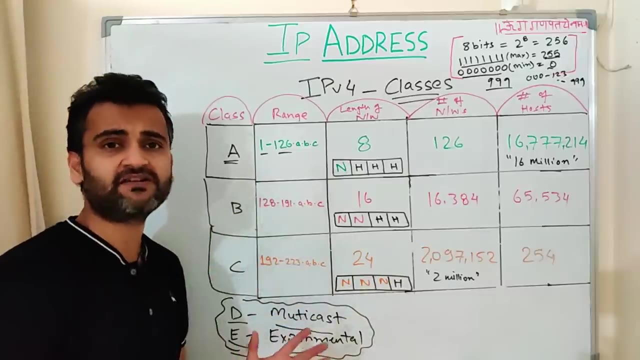 of our whole ip address into different categories. so for class d and class e are not discussed in detail because these are used for multi-class and experimental r d work okay. so we will not discuss these ranges now. okay, but we will discuss these three because you have whatever address you might. 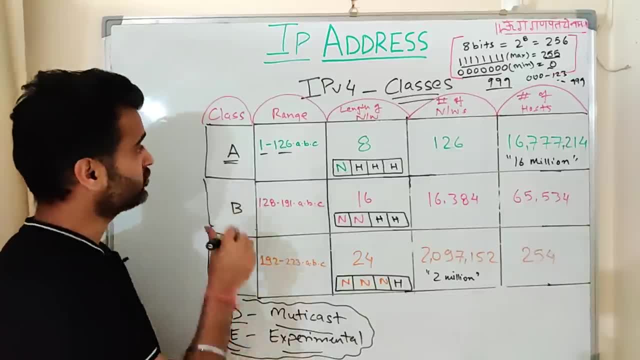 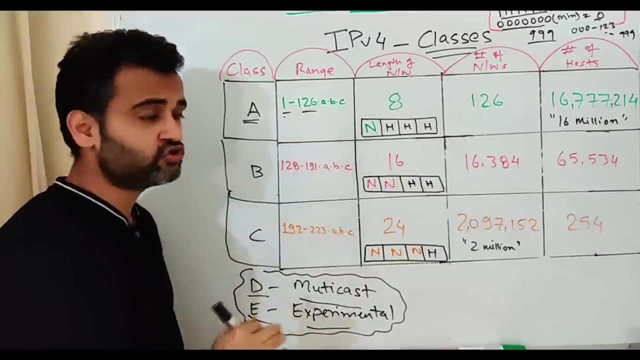 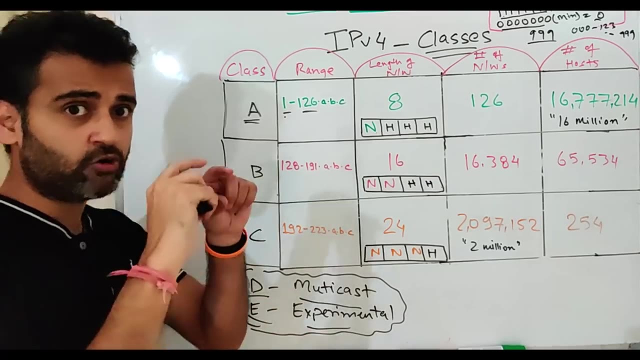 have seen, would fall under these three main categories. so within class a you have all the addresses with the range starting from 1 to 126. so in this particular range, 1 to 126, and in this particular class a, you have, out of four octets of your ip address. remember you have four different. 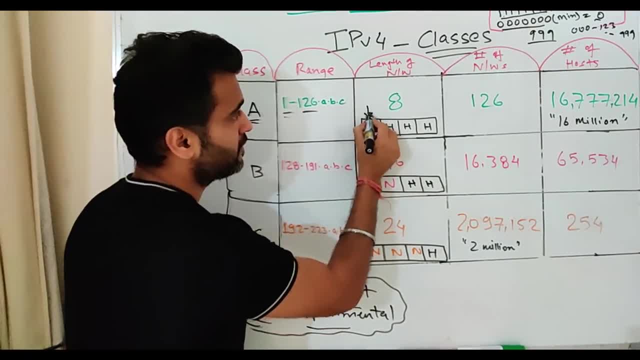 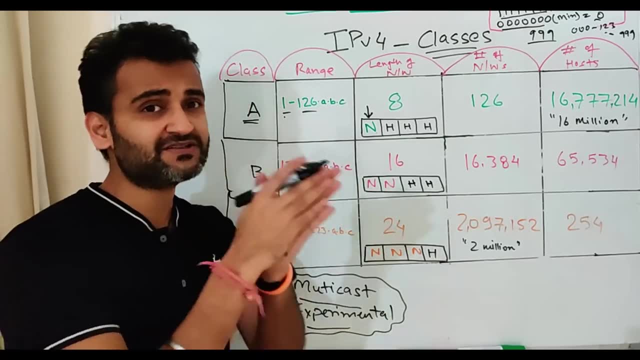 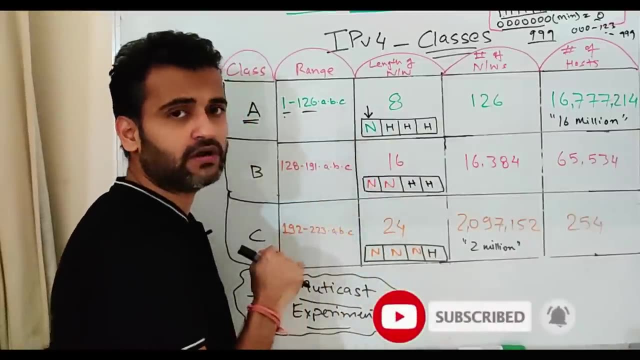 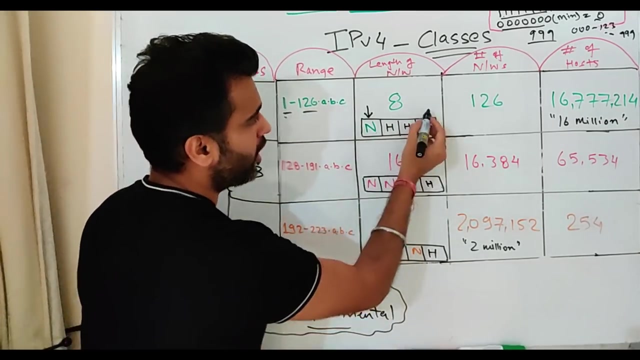 octets you have the first section dedicated to the network. as i told you, ip address is a combination of network ids plus host ids. so in this case you will have uh. the first octet would be dedicated to your uh network and the rest three would be dedicated to your host uh bits. so how many are? 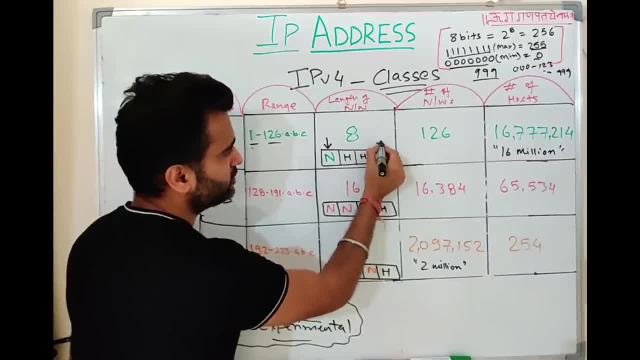 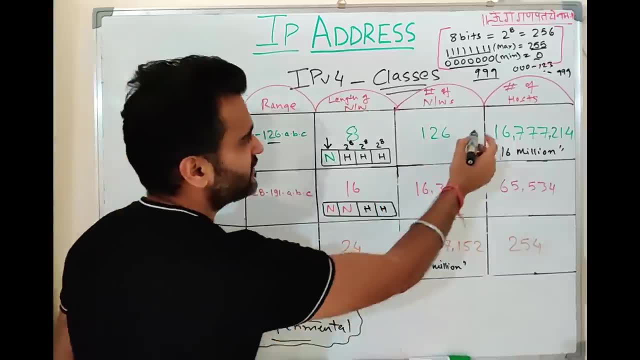 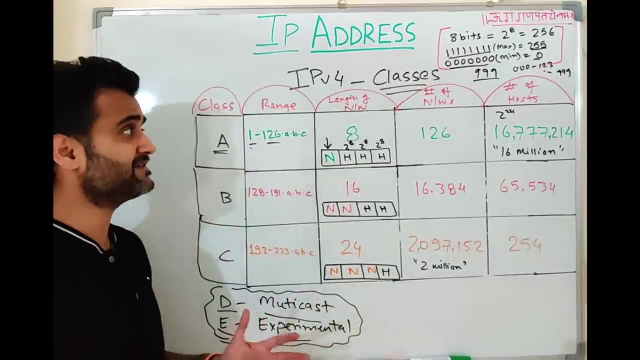 these. so these are, uh, you know, uh, two to the power eight, two to the power eight, two to the power eight, so eventually, these are two to the power 24.. okay, which is, which comes around 16 million hosts. you can understand that in this particular class. 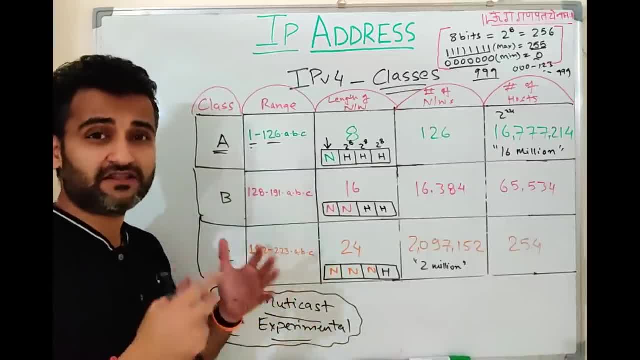 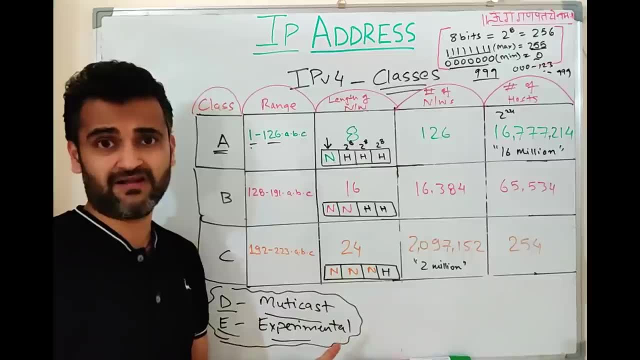 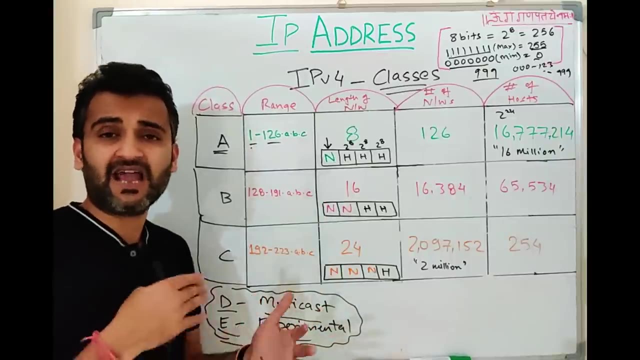 a type of ip addresses, you can have 16 million hosts. that's why these are only dedicated to very, very large networks. it is not given for a mid-level or very small level organization or household. it is always given. so some very famous uh class a addresses are at t ibm and i think 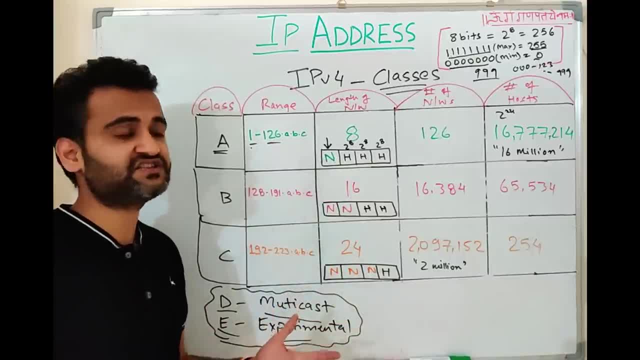 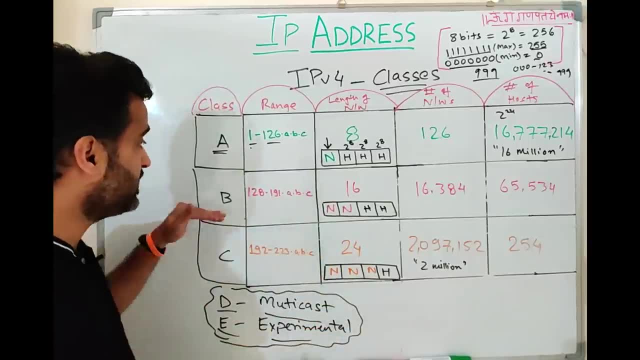 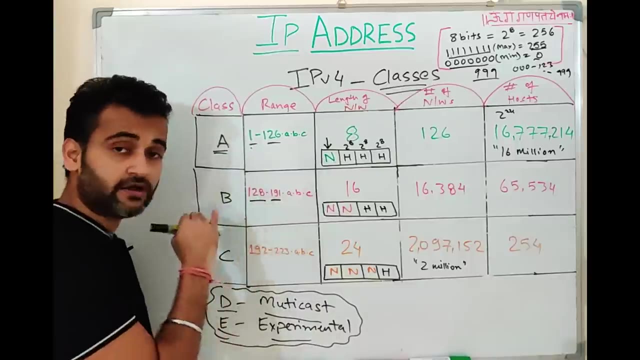 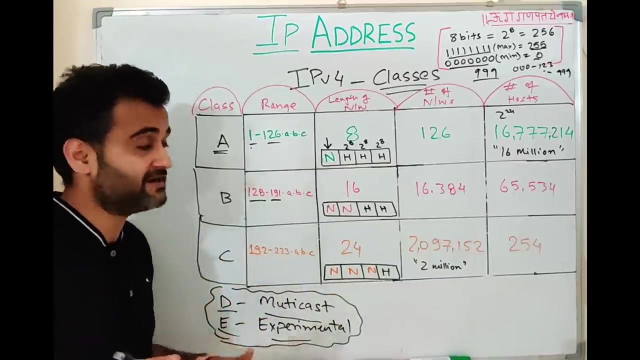 general electrics. all these are large organizations which have already reserved class a, kind of network. so that is, uh, class a, you understood that right. in class b we start from range 128, because we left here one from 126, and then class b address range is from 128 to 191. but hold on, you might have- uh, you know, guessed it that. where 127 went. 127.0.0 range has been reserved for loopback. so you might have seen the loopback id and which can loop back to your same device in. maybe in your windows file you might have seen local host: 127.0.0.0. so that is the loopback. it is reserved for the loopback testing, so that's why. 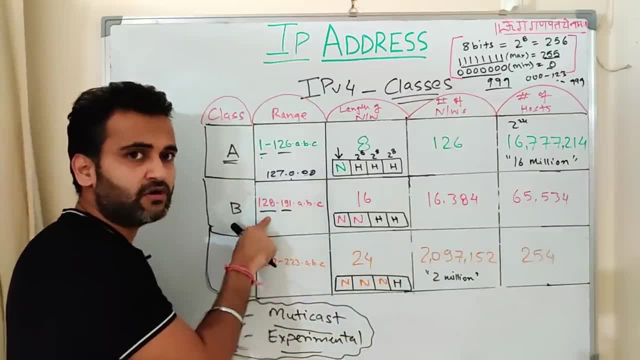 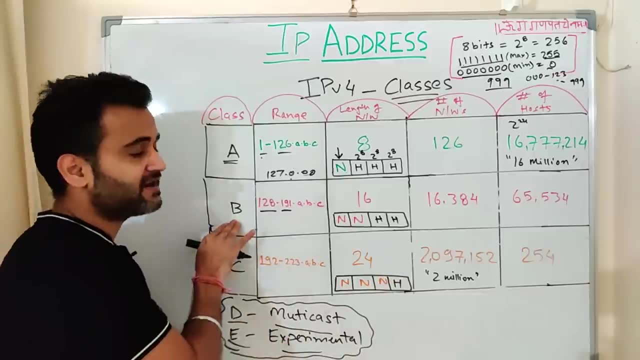 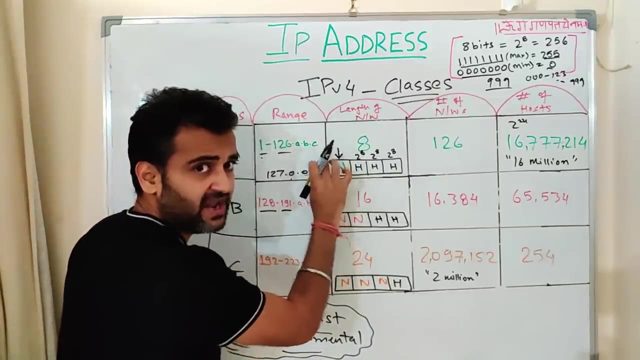 127 range is skipped and we directly start from 128, so in one from 128 to 191. all the ip addresses within this range are considered under class b and in this. so in this particular section we had the first eight bits dedicated for network, but in this we have increased that, so we have two different. 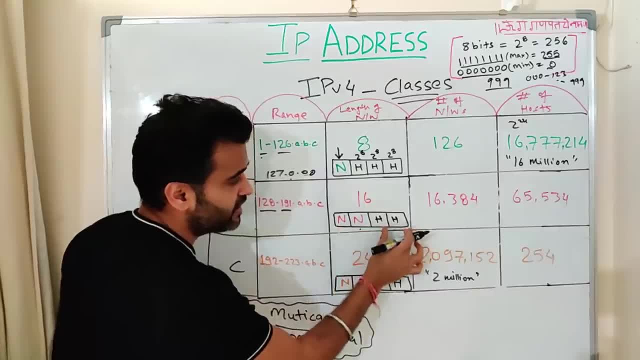 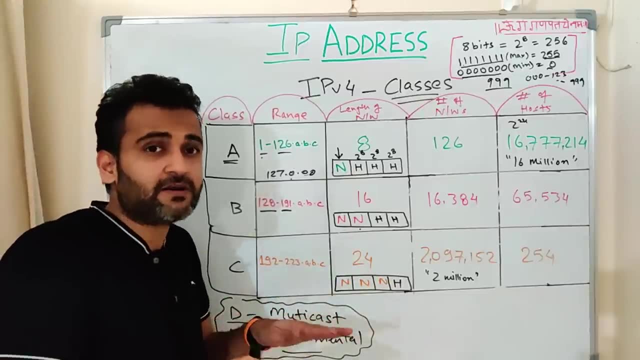 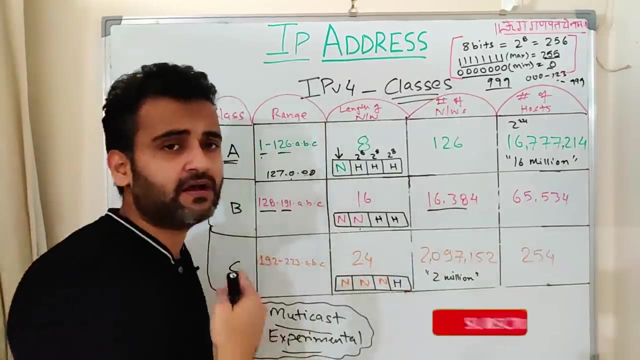 octets, or maybe 16 bits dedicated to network and 16 bits dedicated to host. so this is kind of an equilibrium, is kind of formed here, but not exactly, because here also, you know, you will have around 16,000 different network, okay, 16,000 different kind of networks you can use and 65,000. 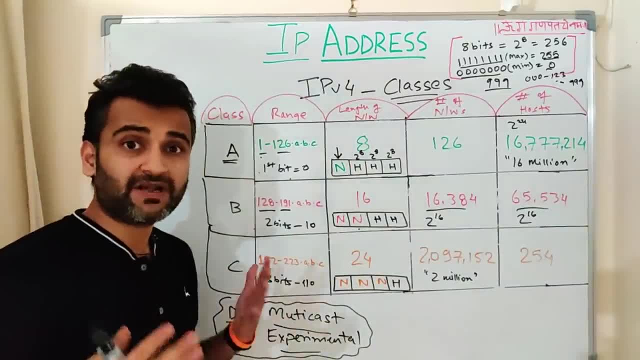 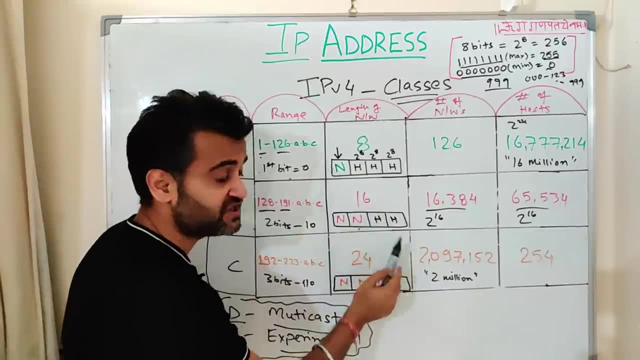 and different host you can use. but a valid question which might be coming in your mind is then: when, when, if this is also, you know, 16 bits and this is also 16 bits, so number of networks and number of hosts, both should be equal, because this is 2 to power, 16, and this is also 2 to the 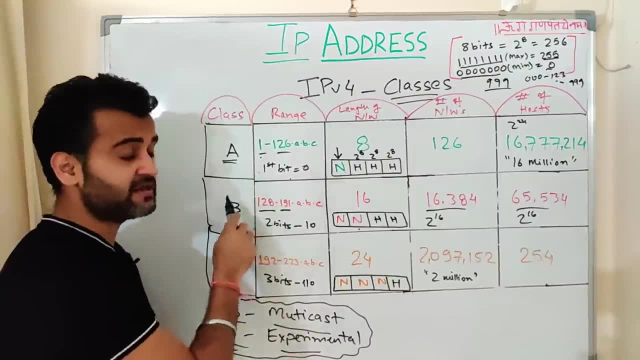 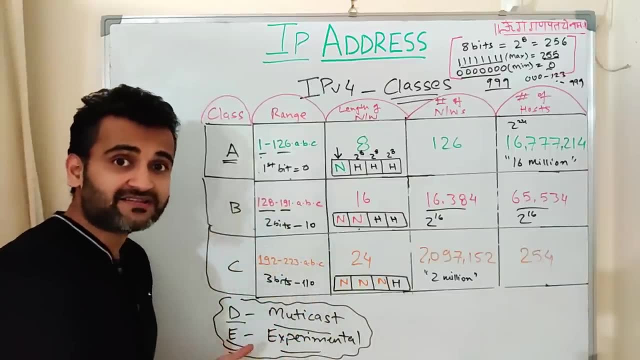 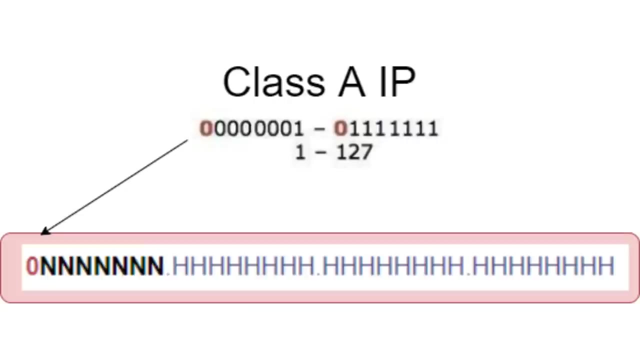 power 16.. but it is not the case because in in case, because, as i told you, the first octet decides which particular class a, class b, class c or class d or class e address it is. that's why some bits of this particular address are dedicated for that. so, in case of class a, your first bit is always: 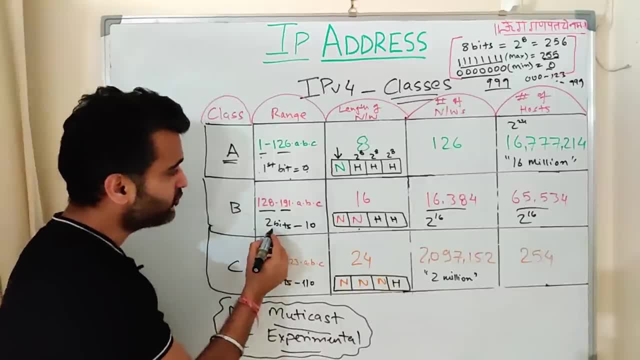 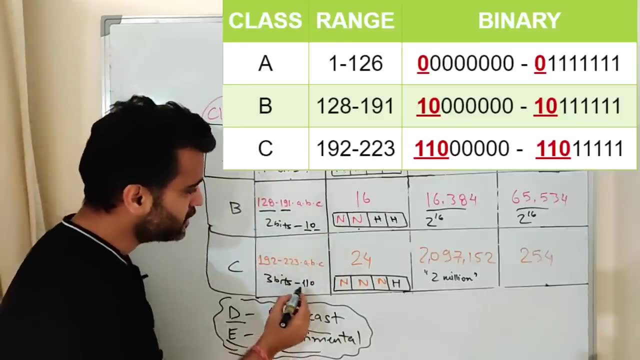 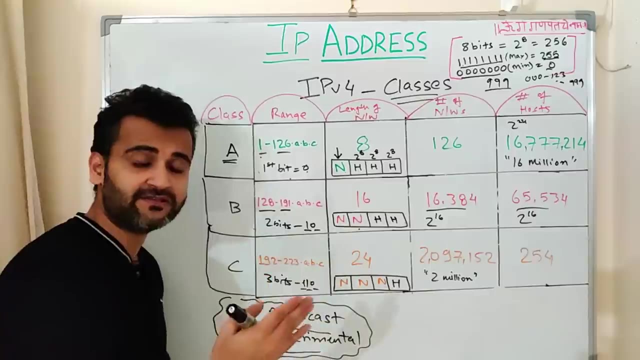 you know, zero. in case of class b, your first two bits out of your first two bits, first bit is one and the second one is zero. and in your class c, your first two bits are ones and the last one is zero. similarly, for class d, your first three are ones and last one is zero. and eventually for: 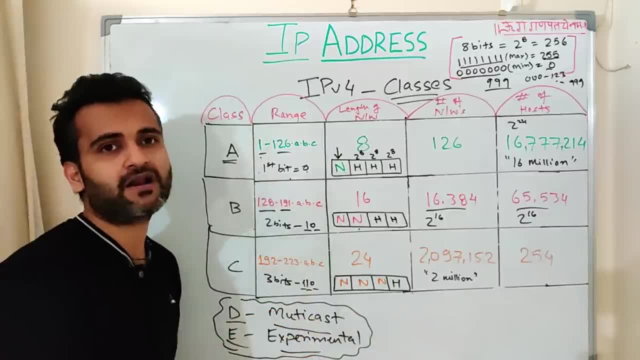 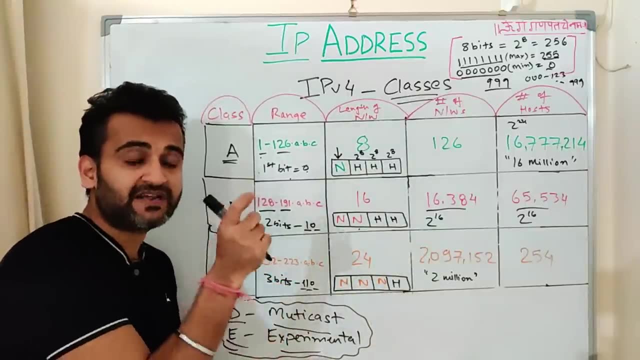 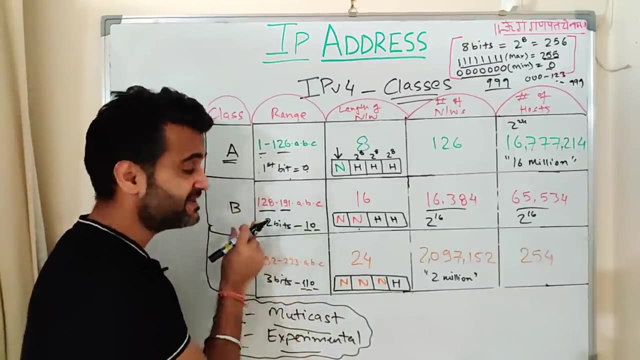 class e. all your four first four bits are one one one. that's why when you are calculating anything for the networks, you have to subtract that dedicated number of bits out of that. so in the in case of class b address, you have two different, you know, bits dedicated for this particular class b address. so what you will do, you have to minus that. 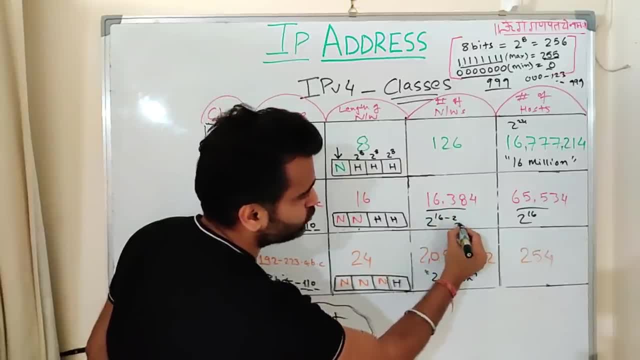 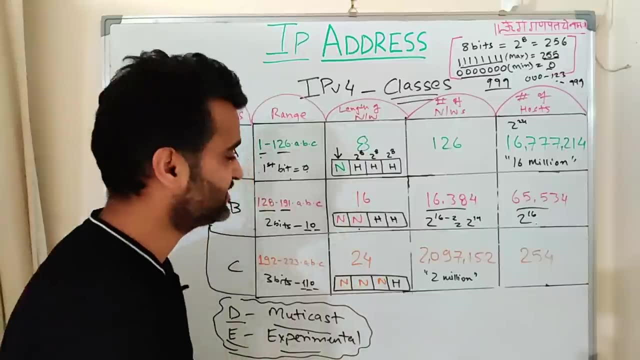 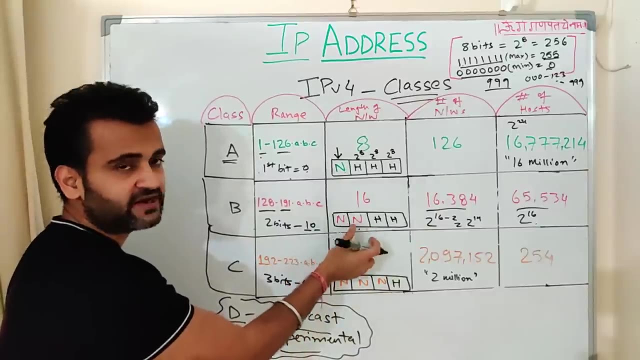 from 2 to the power 16, so it has to be 2 to the power 14.. okay, that's why it comes to 16 384, whereas this remains at 2 to the power 16.. okay, so this is class b address, almost half. first two. uh, you know, first two, the octets are for networks. 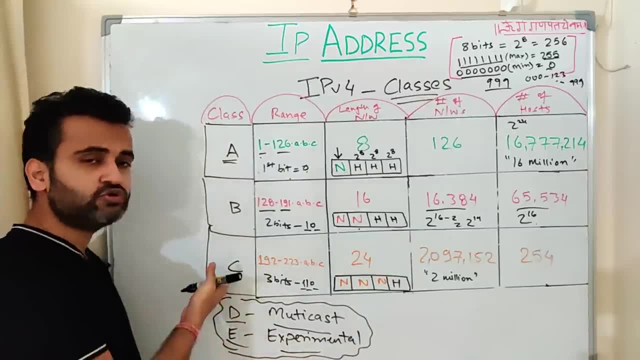 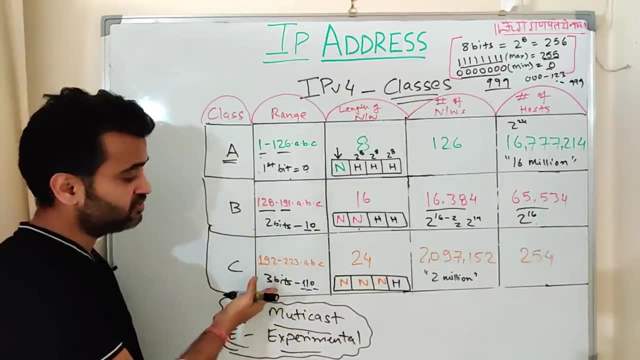 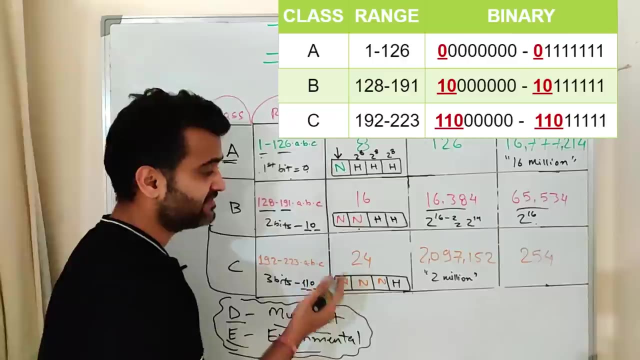 and the second two are for the host, coming to the class c, which starts from the range 192 and ends at 223. this is, again i said, uh, you know the. the first three bits are dedicated, uh, to the network, to for identifying the class of the network, and that's why, here you see, you know you have first three. 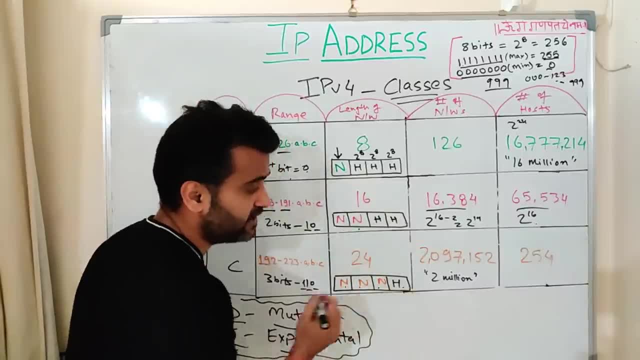 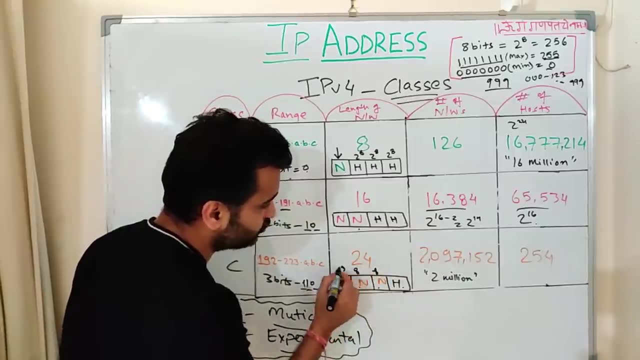 octets given to the network, and then you have the first three octets given to the network and then the last one is uh, given to the host. okay, so in this case the first three are eight, eight, eight. so two to the power twenty four. but it is not two to the power twenty four, uh, it is two to the power. 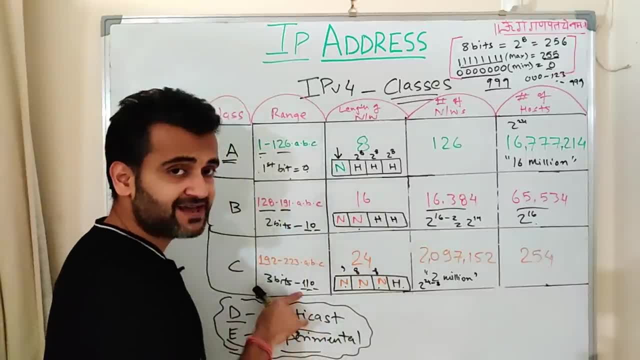 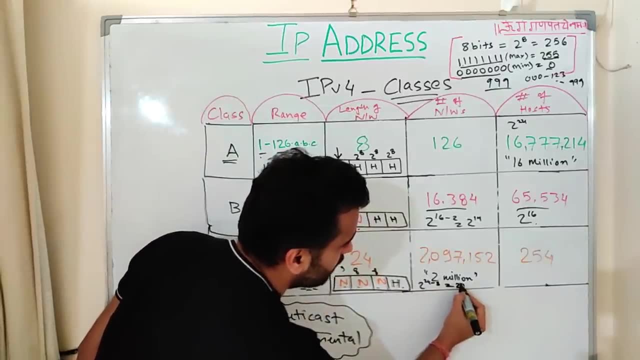 twenty four minus three, because the first three bits are dedicated to identify whether it is a class c network or not. so that's why it comes to two, to the power twenty uh one, which if you will calculate would be two zero nine, seven, one, five, two, which is around two million different. 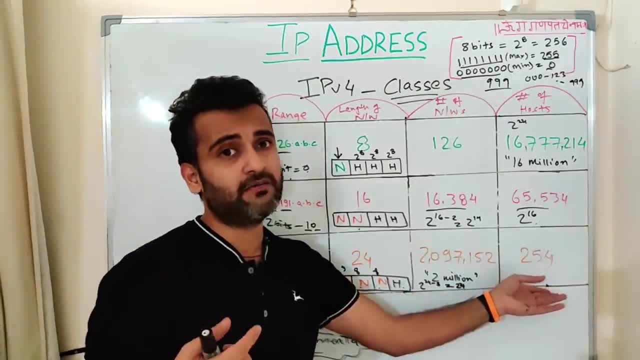 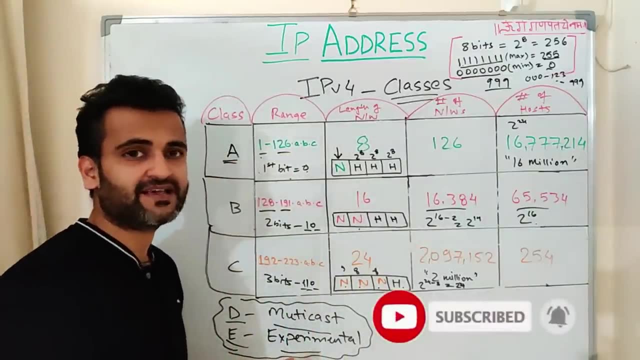 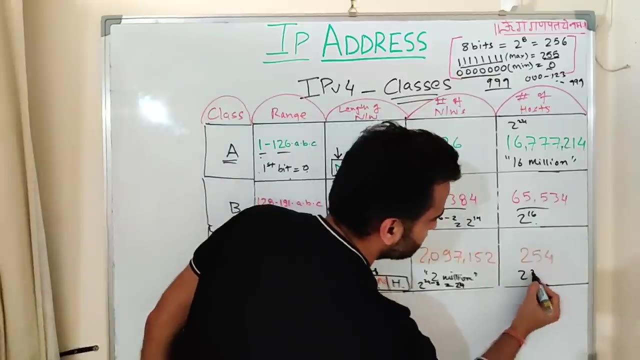 network and ends up with only 254 uh number of uh hosts. okay, and then you know this is the way the network addresses are segregated. okay, and you might also question that if it is, you know, two to the power eight, because only the last octet is there. you know this particular octet is there. 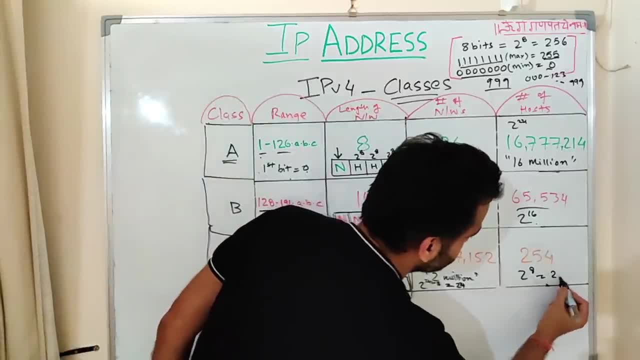 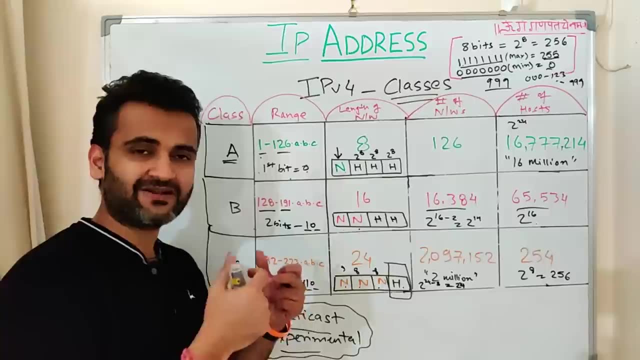 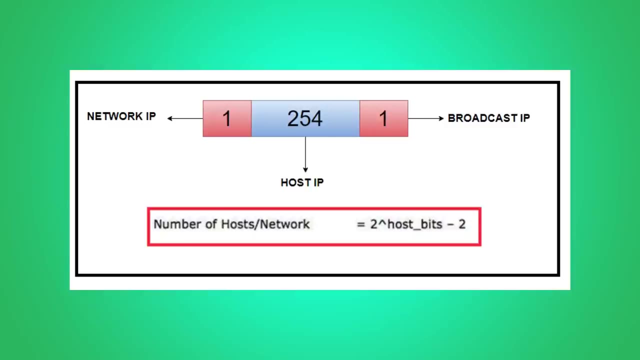 again a good point. so it should be 256. but then always remember that one bit is always dedicated uh to your network and one particular, you know one particular bit is always uh dedicated as a broadcast id. so this particular uh, you know, this particular uh octet or this particular set, 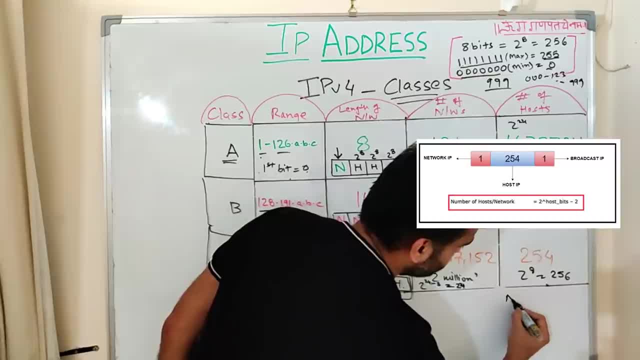 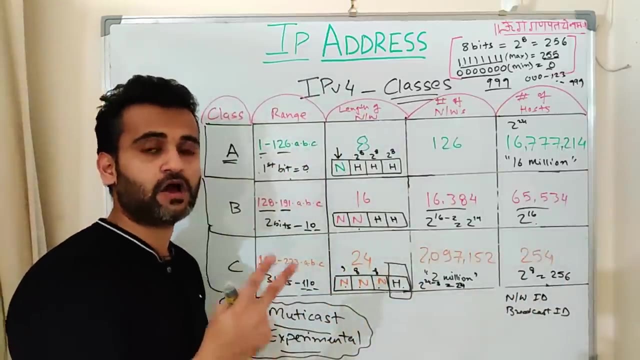 of ip addresses, one particular dedicated uh would be a network id and one could be and one would be the broadcast id. okay, so that's why, instead of giving 256 all to the host, you will have, you know, two minus there will be. i always uh your minus two of the total number of host. 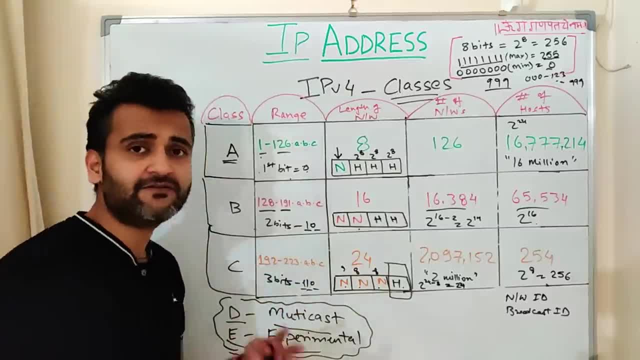 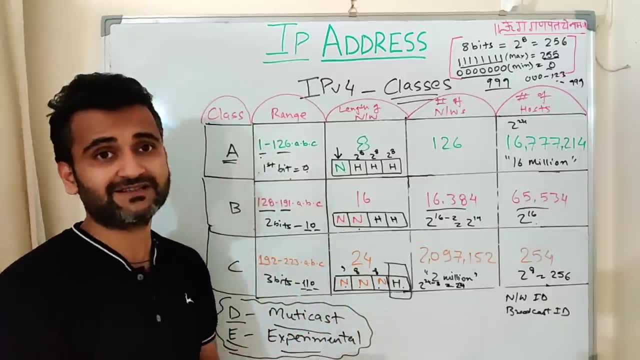 uh, which you can, you know, which you can utilize. so i think these are the three different classes. i have tried to cover it. obviously there are more details to it. you can read it out. i can share. uh, you know some links in the description, but this is the overall concept. so, whenever 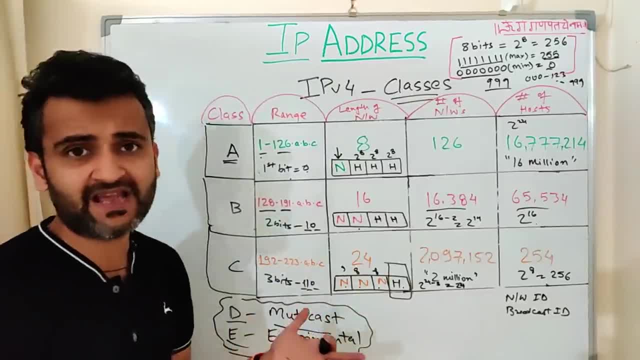 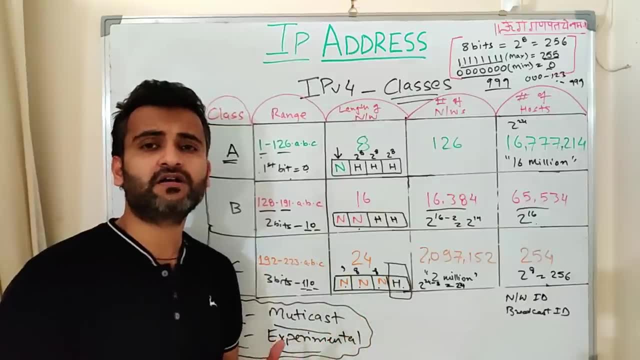 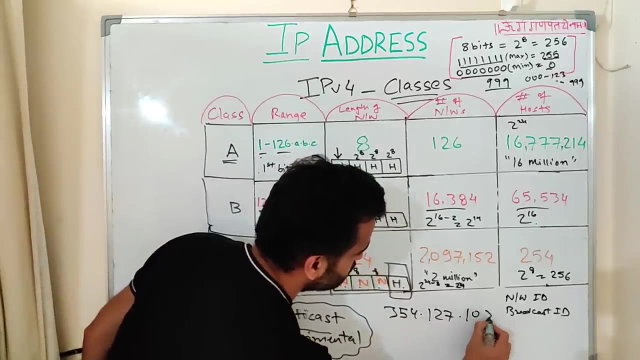 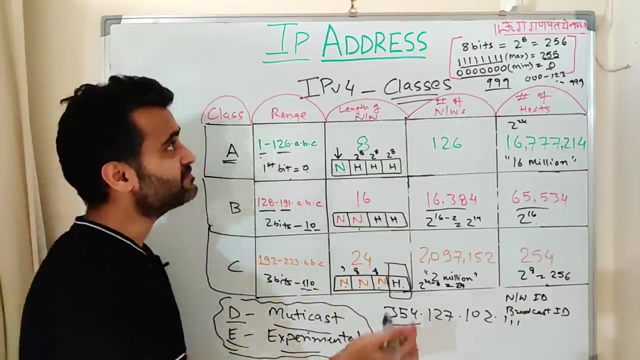 you see any ip address, suppose i just randomly take any ip address and that ip address, uh, you know, could be 354.230.127 something, something so 354.127 or maybe 102 or 111. so then you should straight away say that this is not the correct ip, because the maximum i told 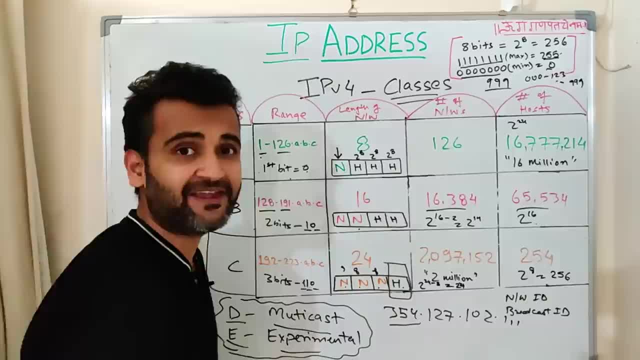 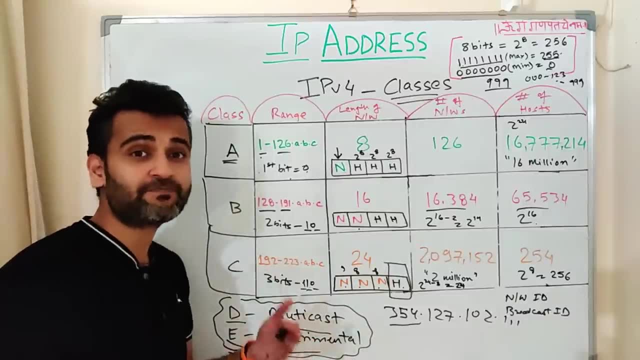 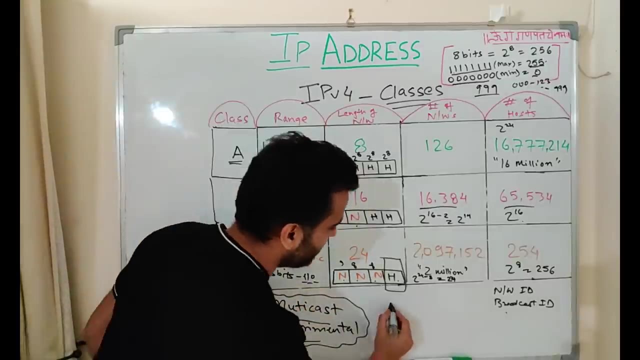 you can, only you can. you can only have up till 255. so first you can see that. okay, no, this is 354, it is greater than 255. how it can be a valid ip. so first thing is, you can now make sure that it is a valid ip. so now, friends, let's take another ip, for example. so suppose i take 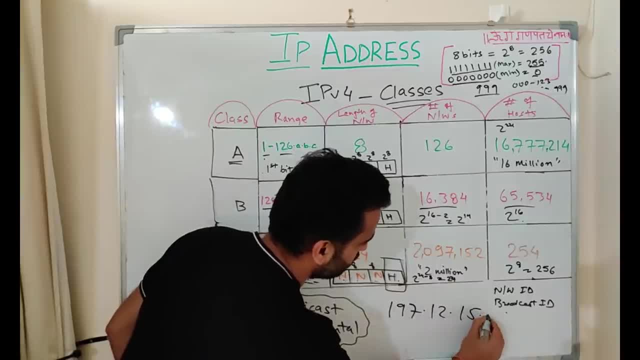 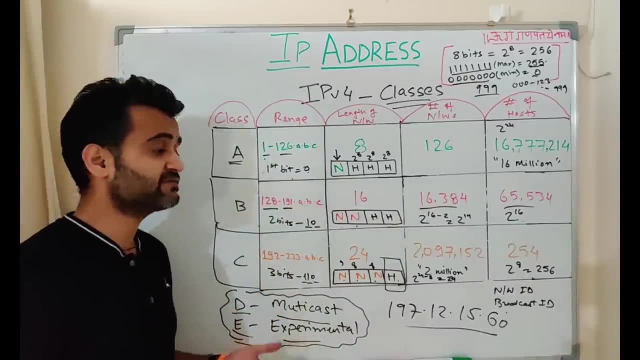 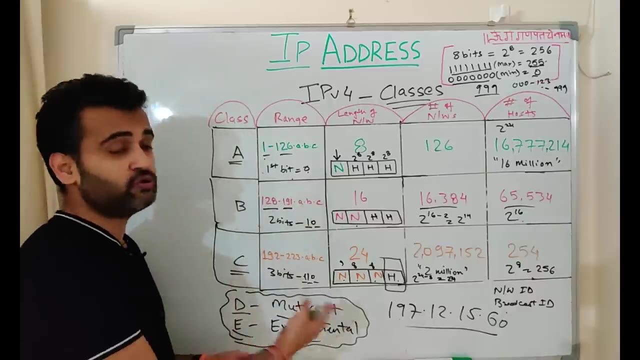 an ip 197.12.15.60. now if you have to see this particular table, you should be able to make out in which particular class this particular ip address falls into. so 197 falls into a class c ip address. so you can take a note of this table. it will help you to identify. 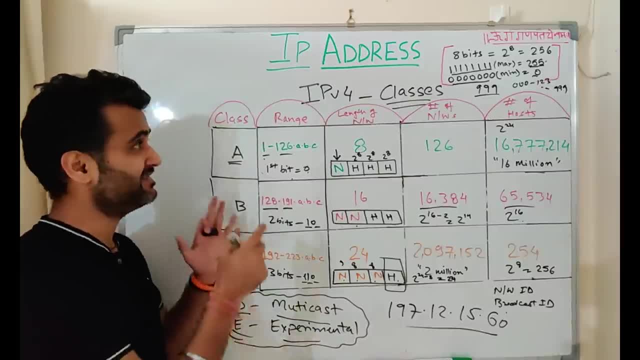 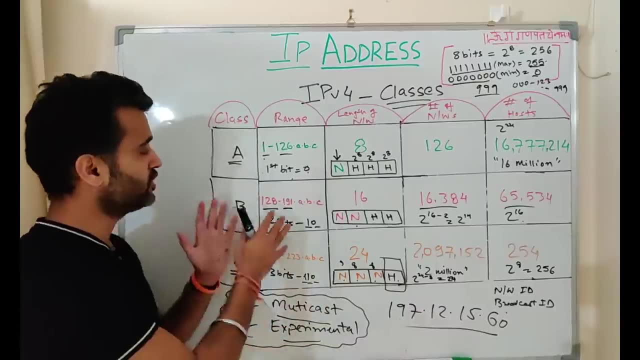 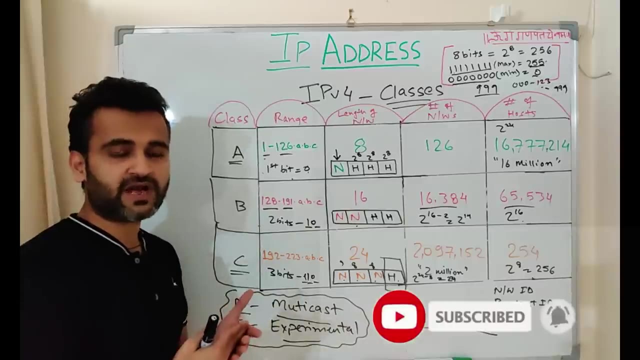 in which particular class and ip address falls into, and And this actually summarizes how one IP v4 classes are distributed and categorized. So now you can see this table and you can identify and understand that while you see a network IP, you should be able to understand how many number of networks could be utilized. 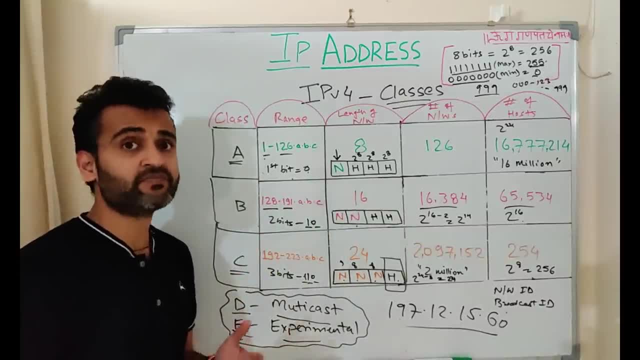 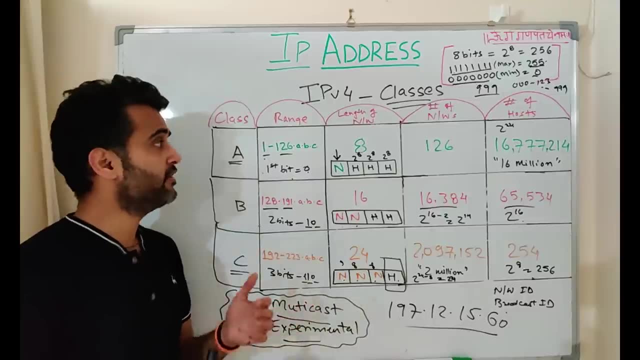 within that and how many a number of hosts can be utilized with that. But there is another concept, which is subnetting, which you might also know. that's a very vast topic maybe we'll cover in some other video, wherein we will understand that these classes are not adequate for the proper distribution of the network. 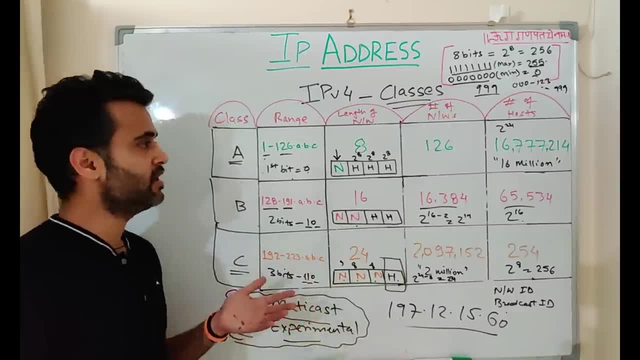 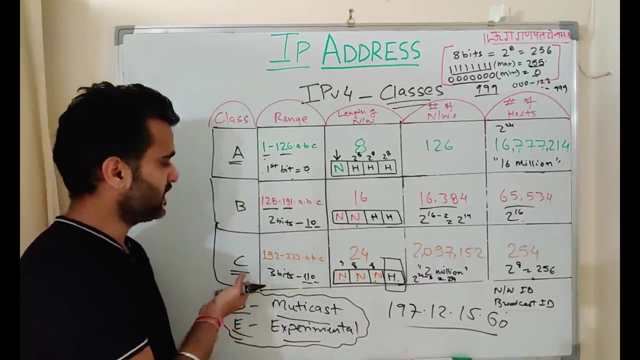 If we go by this, you know this- we would be exhausting our network bandwidth quite easily, because this is not an ideal case. Suppose you have a small network requirement, then in which particular class you would fall. Suppose if you want only 50 hosts, maybe you take up, you want to take maybe class C or 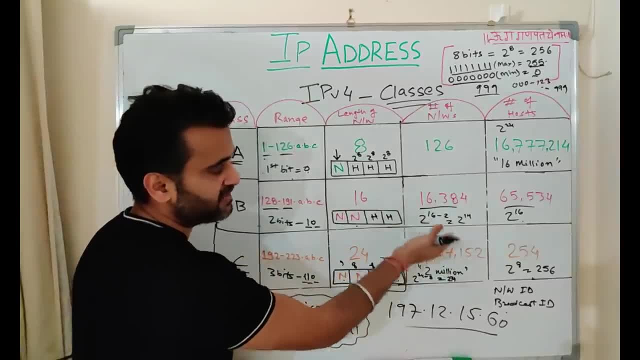 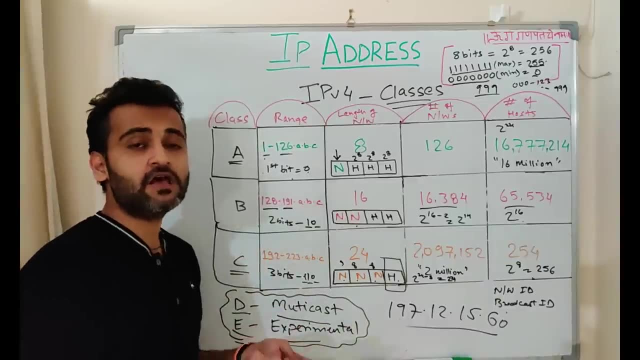 class B. So just understand how much number of networks And you know, hosts are there. So you have to maintain that balance and that balance cannot be maintained by simply using these classes. You have to further use concepts like subnetting to utilize these IP address in different manners. 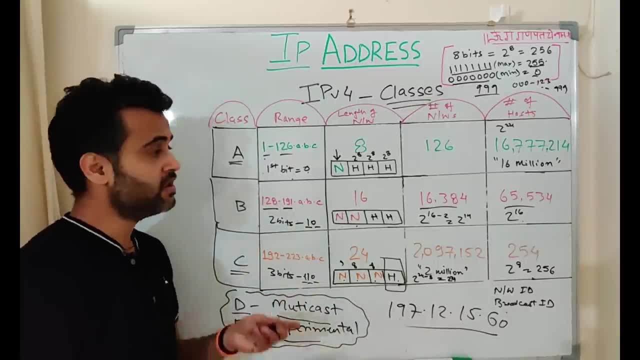 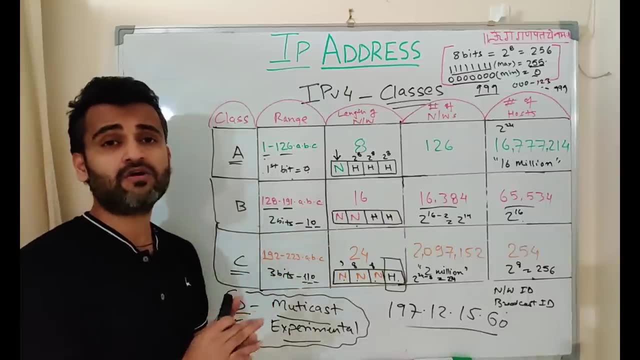 and you know, distributing one network into multiple sub networks. So that may be for another video, but for now this should be enough to get you going. So in the next section, let's now understand what is the difference between a public IP and a private IP. 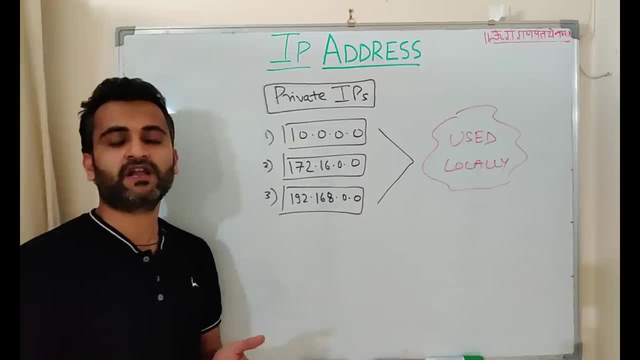 So, friends, What is the difference between a public IP and a private IP? So understand this, guys, that a public IP is always there, over the, over the internet, over the network. whenever you want to identify a device uniquely, you need a public IP for that. 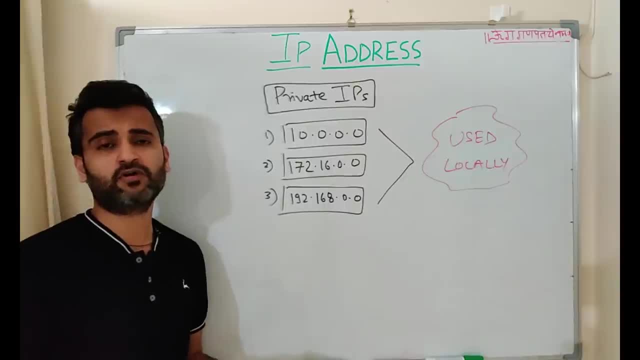 But what, what? what if you want to use IP addresses for your local usage? suppose, within your company you have your local area network or land and you want to distribute IPs for that? you do not need, you know, you do not need the whole IP range which is reserved for public IP, for. 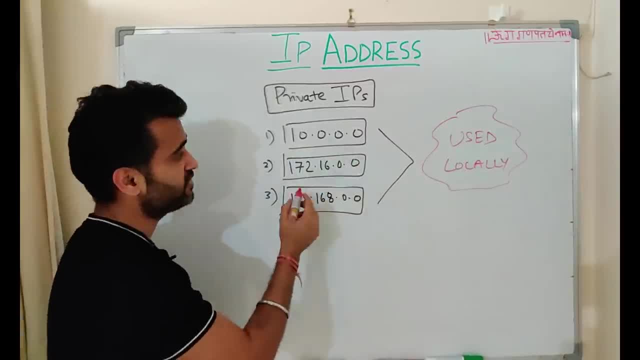 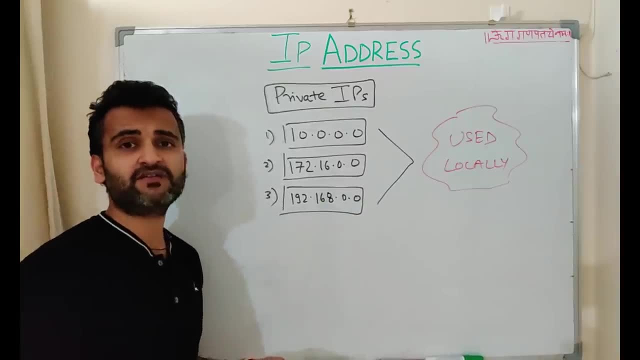 that That's why we have this dedicated range: 10.0.0, 172.16.0.0, 192.168.0.0. so whichever IP addresses you see within the network would fall within this particular private IP range and then 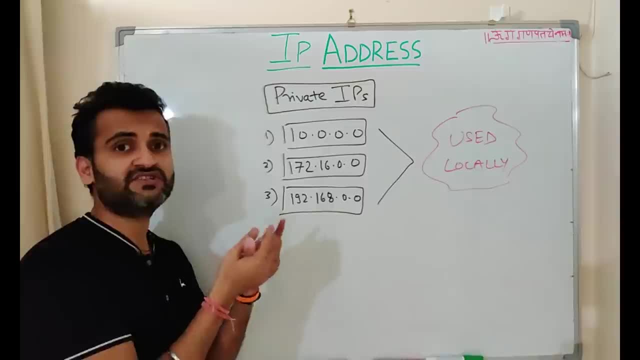 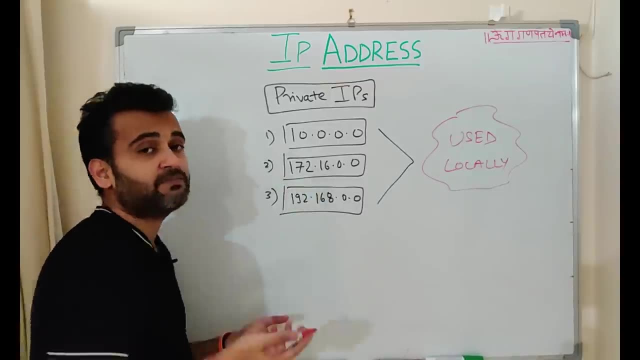 that is the case, two different networks could have the same IPs, because these are only for private and the local use And that's why it can happen that two different networks you know might have the same IP address. Most of the time, It is that you will have these IP address shared internally among different organizations. 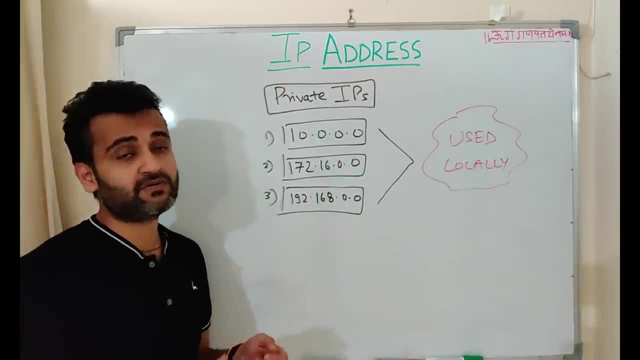 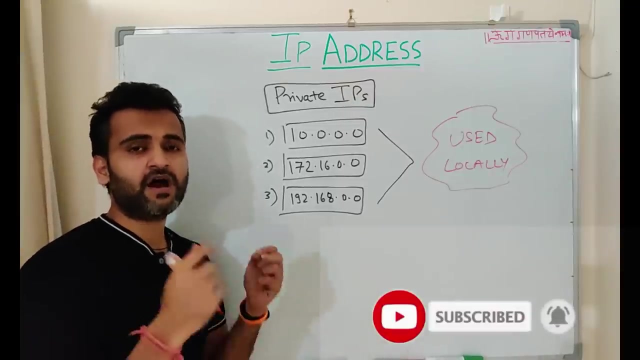 This is only for local use. obviously, when you'll go to the public network, then you have to fall back upon your public IP ranges, which we discussed previously. So this is private IP and this is the difference between public and private IP. Now, finally, let's understand our final section, wherein we understand what is the difference. 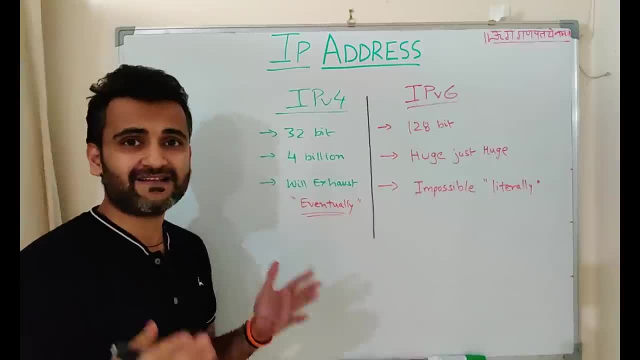 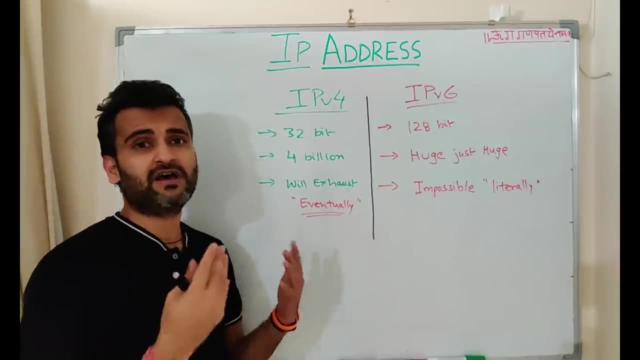 between IPv4 and IPv6.. So Now, at the last part of this video, let's understand what is the difference between IPv4 and IPv6.. So IPv4 was the version which came more than 20 years back in the world of networking and 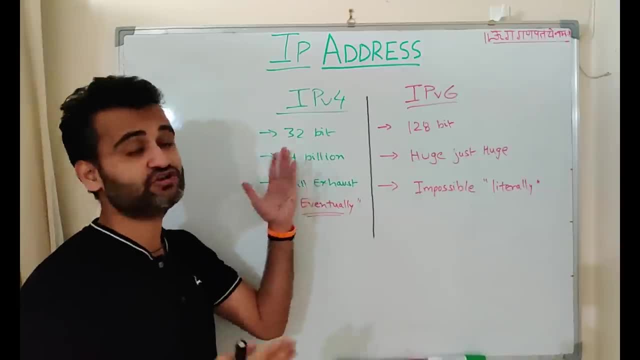 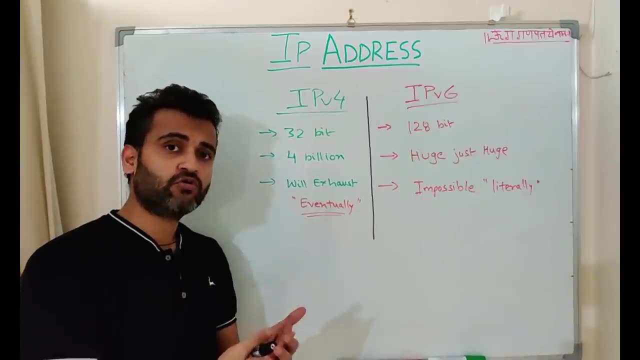 it has been continuing since then. But you have to understand that this is eventually a 32-bit IP address and a maximum of 4 billion IP addresses could only be utilized. So you know the researchers knew that. you know this would exhaust, so they always wanted. 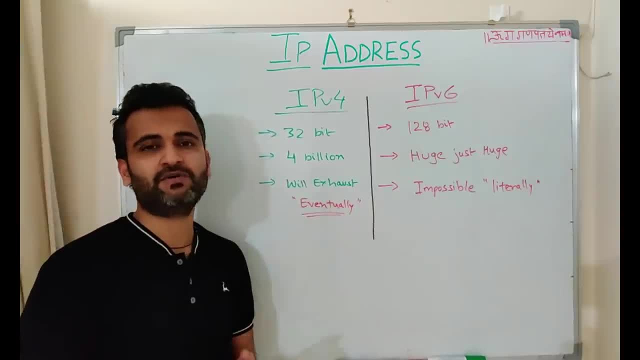 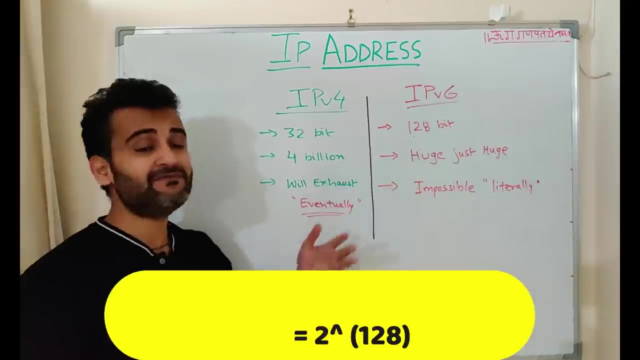 to move to a version of IP where you could have enough IP Addresses to cater to the future demands. So that's why they came up with a 128 bit of IP address, which is called as IPv6.. In comparison to IPv4, which is a 4 billion number, IPv6 is just huge. I cannot even tell. 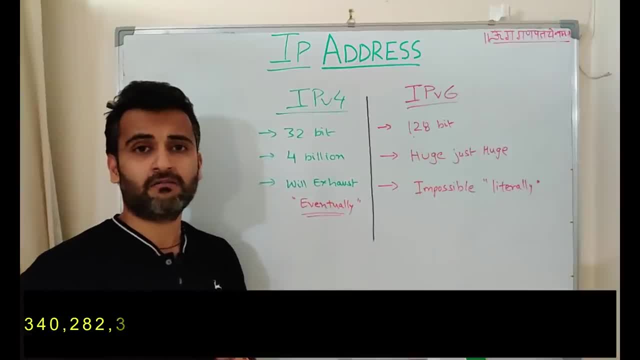 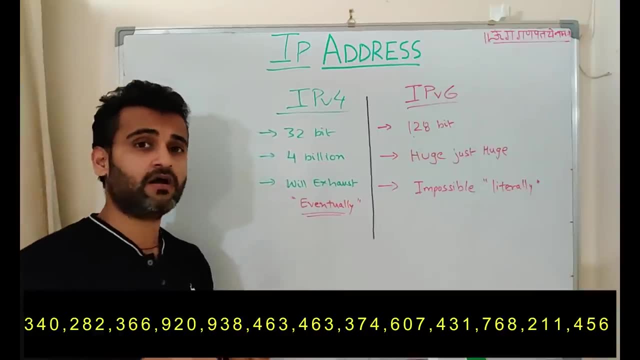 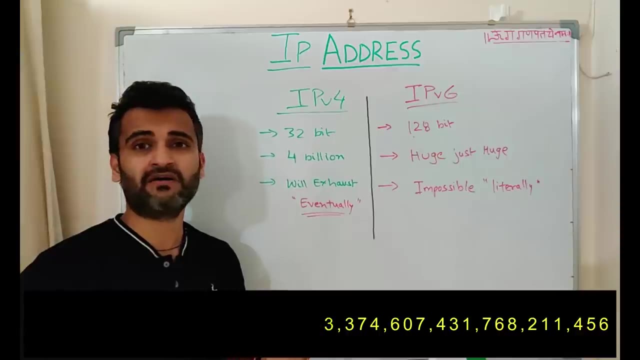 you the number. I maybe I'll show you somewhere on the screen while I'm talking, but literally it is. it is so huge that if I just have to give you an example, if you have, if you are assigning thousand different unique IP addresses Per second, then it would take you- you know- billions of years to exhaust even 1% of the. 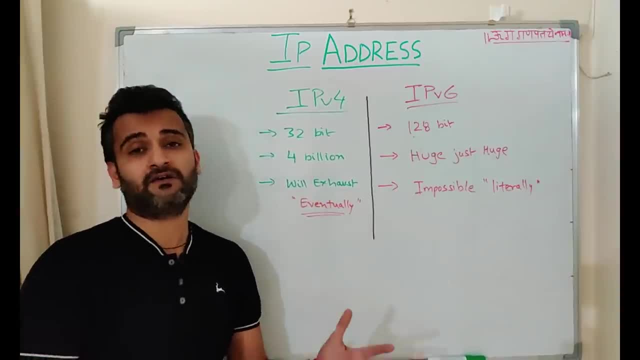 total IP address. I am not joking, guys, This is what I have read and you can maybe cross check that. I'll maybe give you some links in the description as well. So literally this is impossible. to you know, exhaust IPv6 it is. it is just a huge in number. 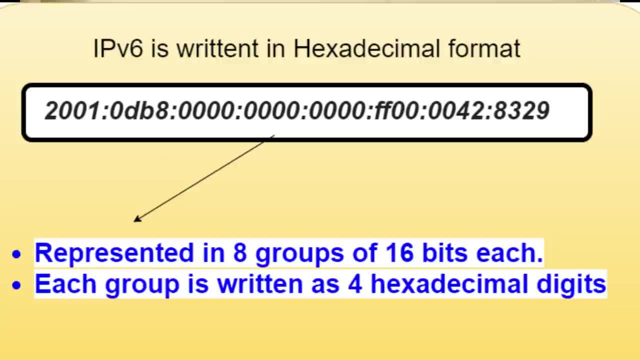 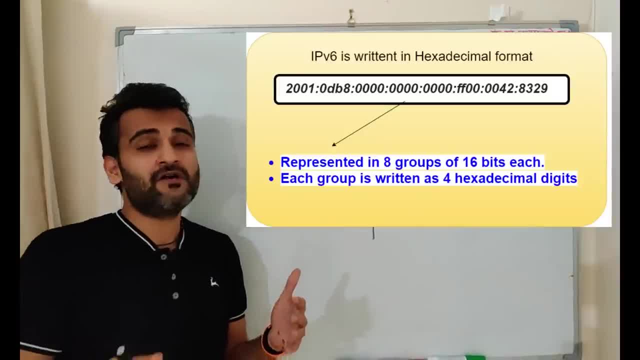 but IPv4 will sooner or later- you know will- get exhausted. But the irony is all this was forecasted in around year 2004, when you know, when everyone thought that you know the maybe in 2-3 years of time, IPv4 just go away. 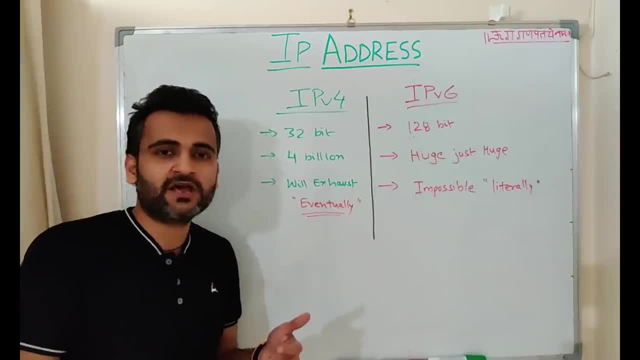 But with the current advent of advancement of networking concepts like subnetting and everything, we have sustained IPv4 till date and today also. we are not sure whether, and exactly at what time, IPv4 will get exhausted, But most of our devices, Most of our computers, 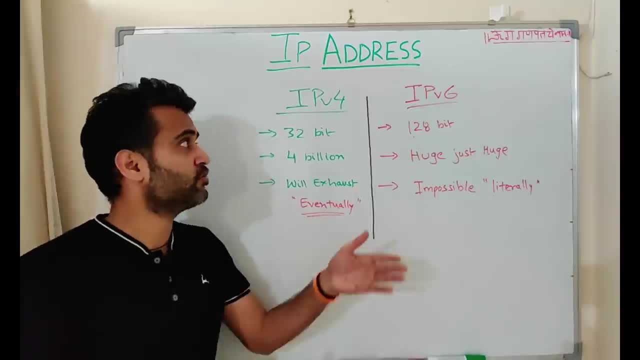 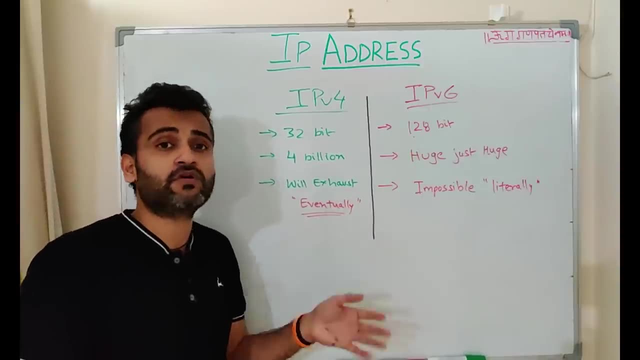 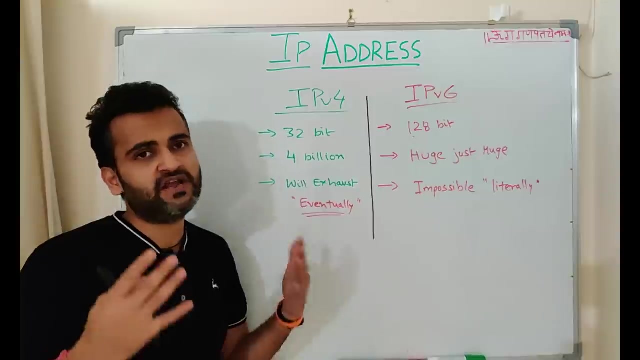 Most of our computers and softwares and hardwares are now supporting IPv6, but the transition is very, very slow, So we really don't know when eventually we will cut off from IPv4 and eventually move into IPv6. but yeah, that is there and as and when we need it, we have to, you know, move. 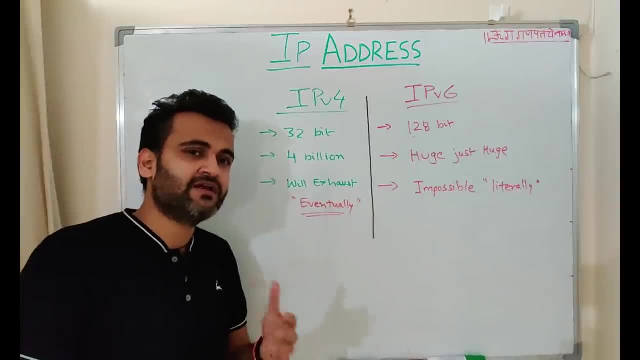 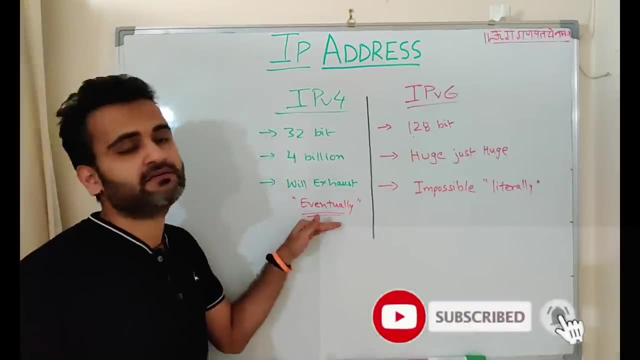 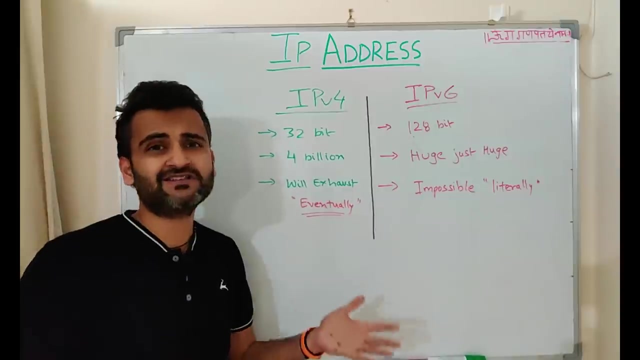 Obviously there are some compatibility issues and that's why you know the absorption rate of IPv6 is very, very slow, But eventually This will exhaust. IPv4 will exhaust eventually and then we will have no other option but to move to IPv6.. So this is a very, very quick difference between what is an IPv4 address versus what is an. 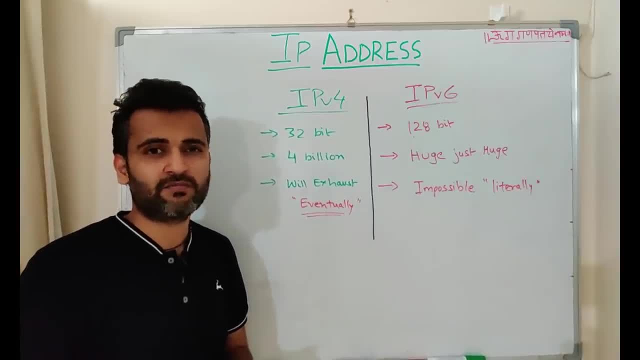 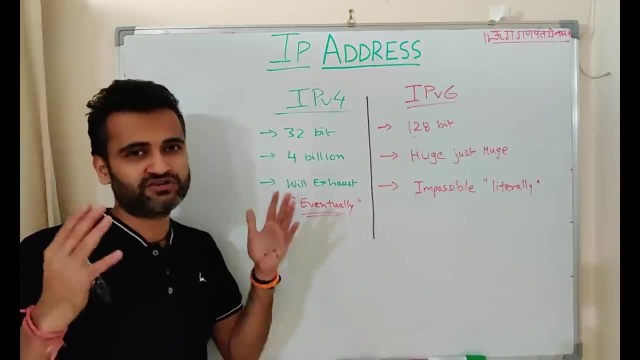 IPv6 address and how these are different from each other. So, guys, I think this this has been a very long tutorial, but I hope you enjoyed it. So, just to recap, we started with the basics of binary, then we understood the structure of an IP address. 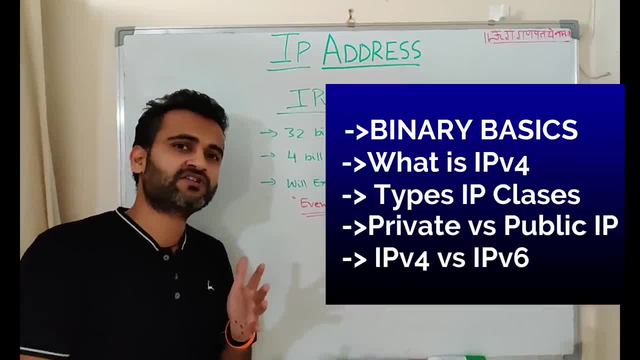 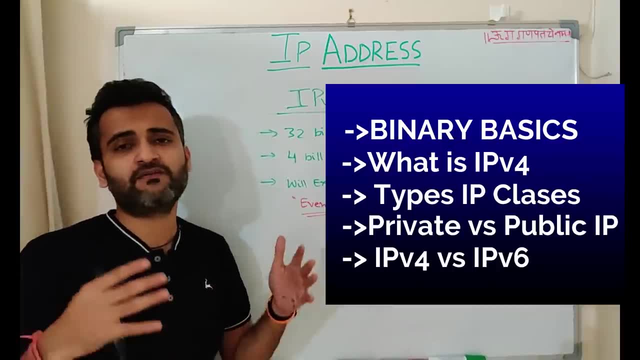 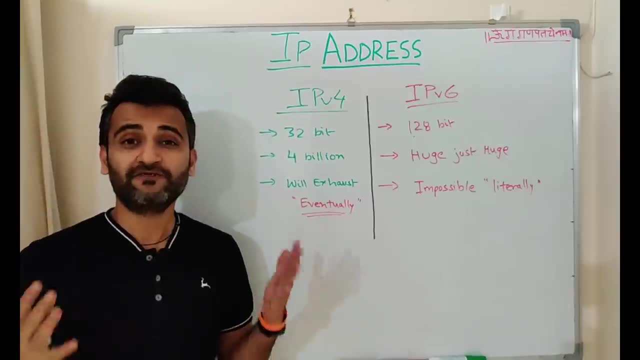 How IP address works, How IPv4 address is structured. We also understood various classes under which IPv4 address is classified. Then we moved on to understand what is a public IP, what is a private IP and eventually now we know what is IPv4 versus IPv6. 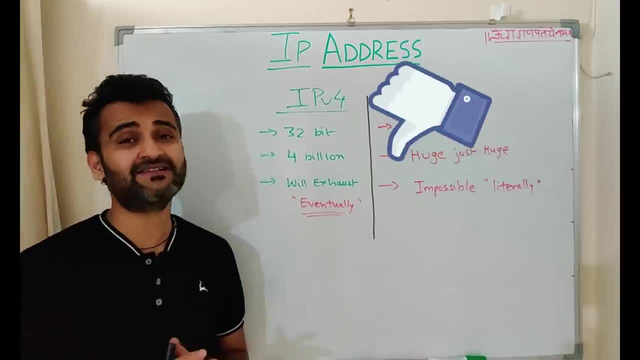 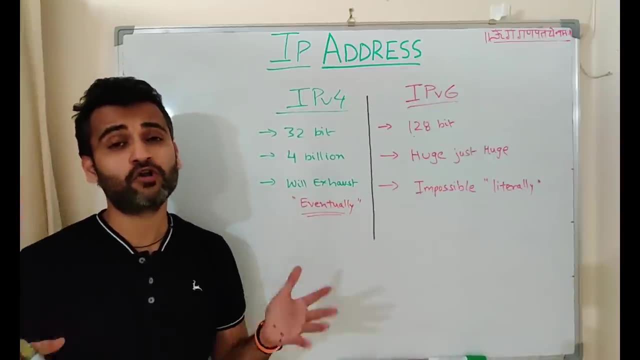 So, friends, I hope you liked this video and if you did, please hit the like button, Please hit the subscribe button to get more videos like this. and also let me in the comment section below, what you would want to learn next In the field of networking or any other field of IT. 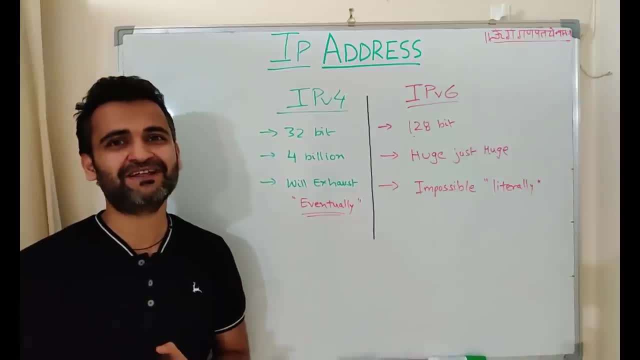 So until then, please keep supporting, please keep hitting the likes and, yes, keep hustling. Bye for now. 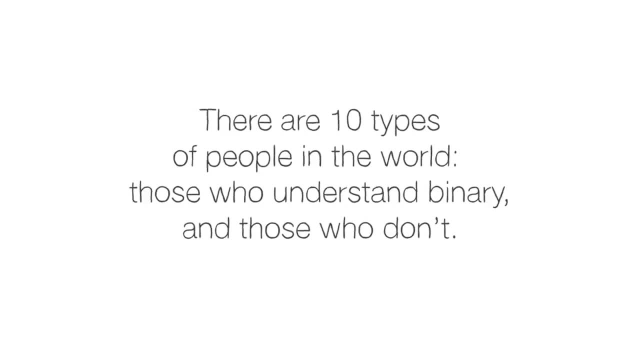 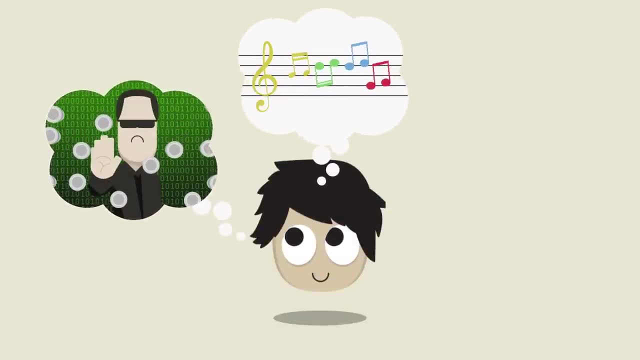 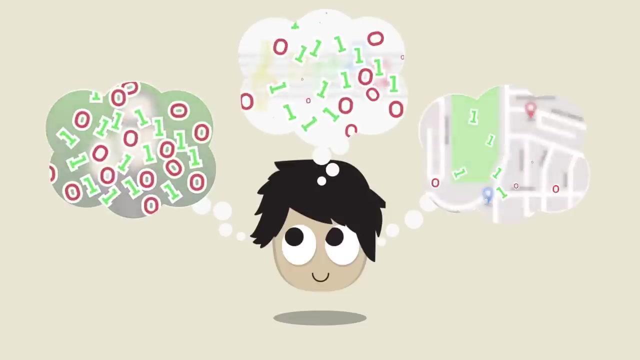 Imagine trying to use words to describe every scene in a film, every note in your favorite song or every street in your town. Now imagine trying to do it using only the numbers 1 and 0. Every time you use the internet to watch a movie, 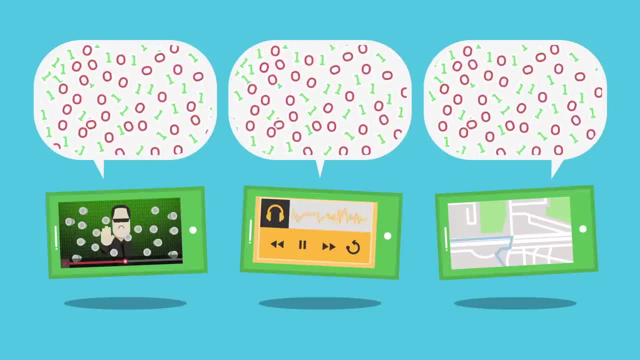 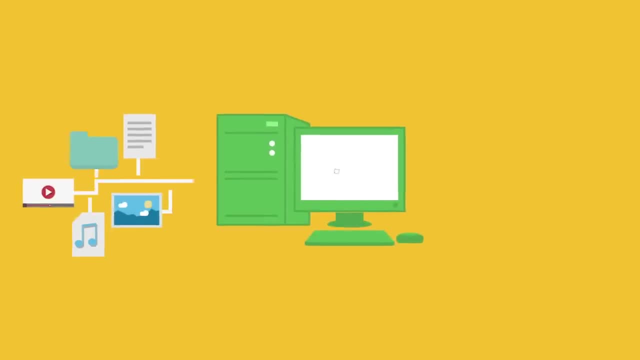 listen to music or check directions. that's exactly what your device is doing using the language of binary code. Computers use binary because it's a reliable way of storing data. For example, a computer's main memory is made of transistors. 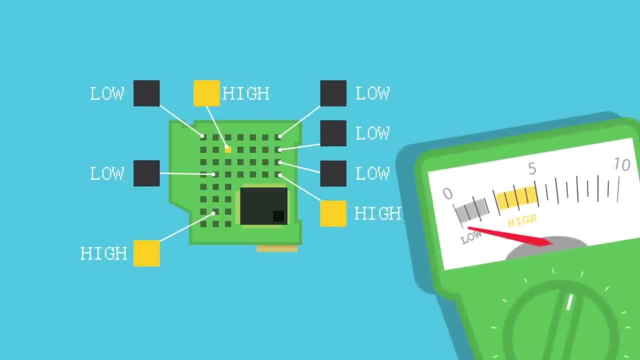 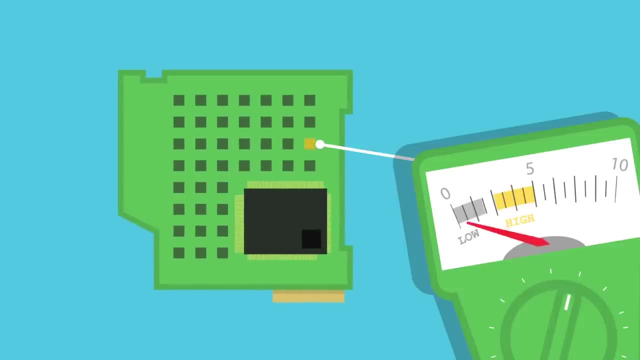 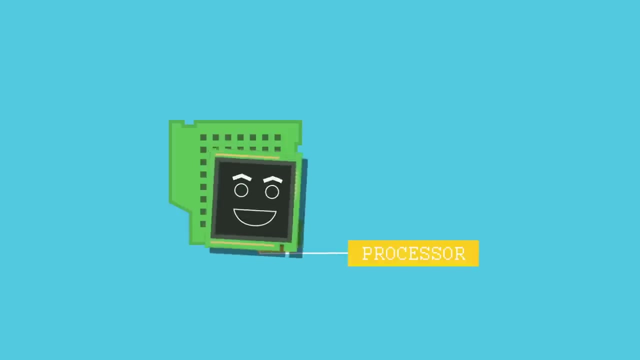 that switch between either high or low voltage levels, such as 5 volts and 0 volts. Voltages sometimes oscillate, but since there are only two options, a value of 1 volt would still be read as low. That reading is done by the computer's processor.